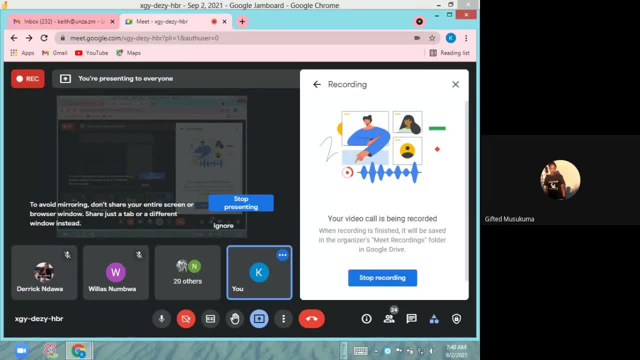 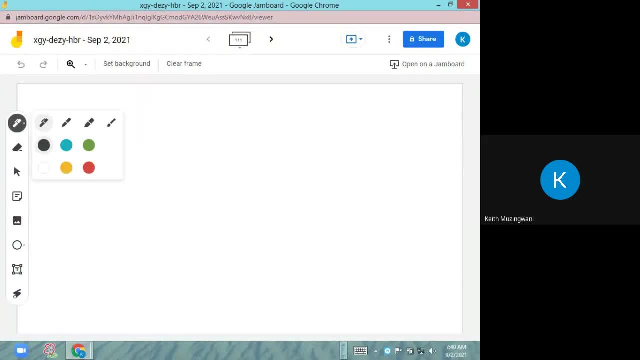 Okay, so we are, we have started looking at. we are looking at methods, methods of differentiation, And we did the first method. Now our second method is power rule. If you understand this rule, you will know that all other rules becomes a given thing. 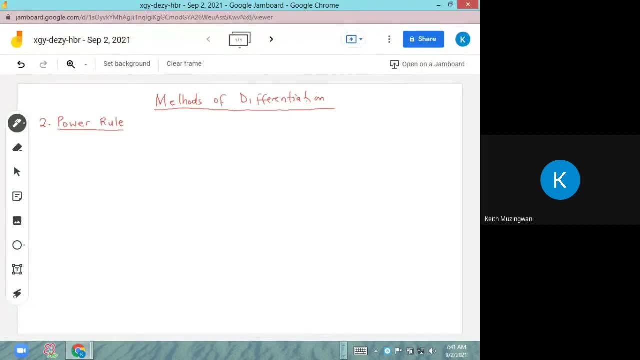 Because it will appear in every other rule. So if, if y is equal to x to the power n, then the derivative of y is equal to n, x to the power n minus one. This is called power rule, Even if we had something like: 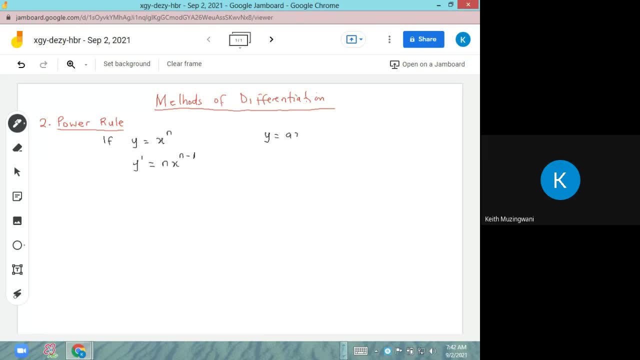 a, x, n. the derivative is going to be a multiplied by n, x to the power, n minus one. That's power rule. Second and third, we look at chain rule. This is a summary of all the rules. 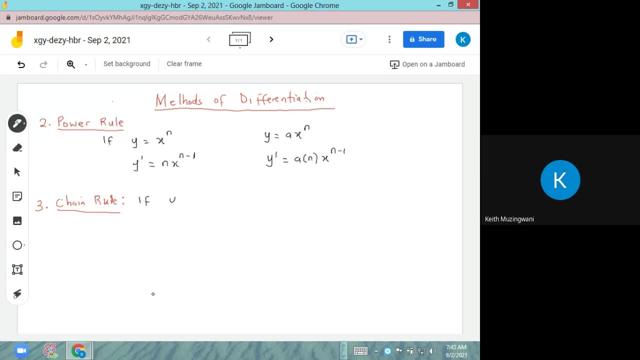 So if y is u to the power n, where u is a function of x- I told you it was a question- where u is a function of x, then the derivative dy dx is equal to. 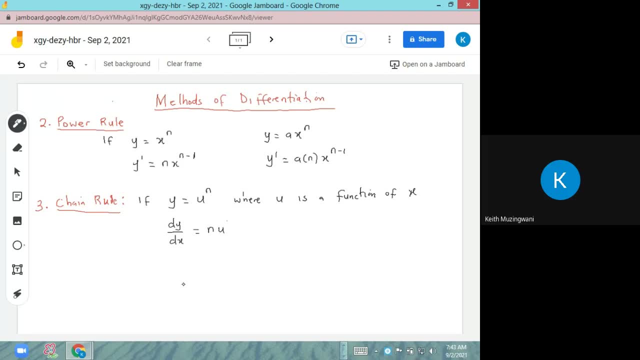 n, u to the power n minus one multiplied by the derivative of u with respect to x. This is called chain rule Or product product: u, If y is equal to u multiplied by v. where 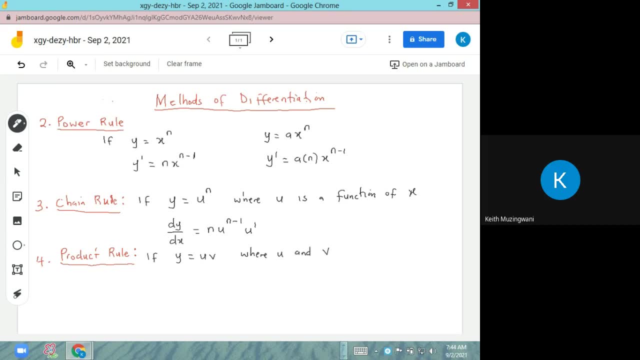 u and v are functions of x, then dy dx is equal to u prime multiplied by v plus v prime, v prime multiplied by u And then five quotient rule If y. 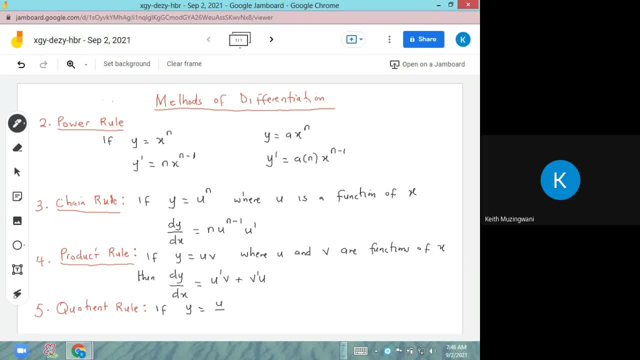 is equal to u over v, where u and v are functions of x, then dy dx is going to be u prime v minus v prime u over v, squared. This set of four rules. 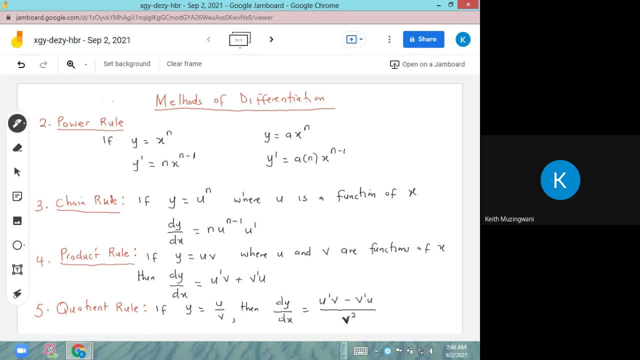 plays a very, very important role in calculus. Without power rule, you cannot have chain rule, You cannot have product rule, you can't have quotient rule, Because you have seen that every other rule is going to be using. 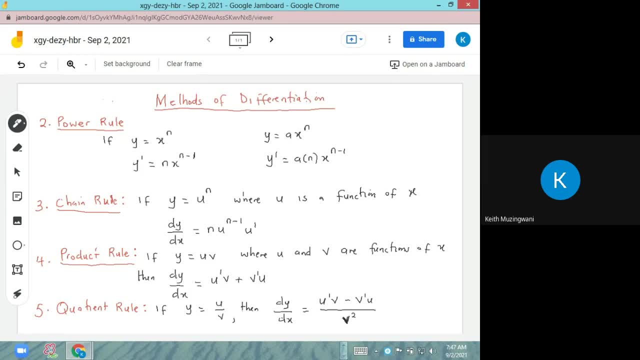 power rule. Excuse me, sir, I just wanted to find out on the chain rule, because the first part where it's saying n? u to the power, n minus one, it seems to be it. 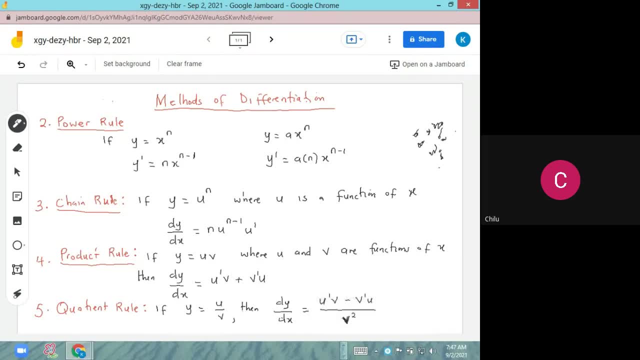 it has been. they've found the derivative of that, that that function And also the? u seems to have that cap prime thing. Does it mean the u also? you need, you need to find. 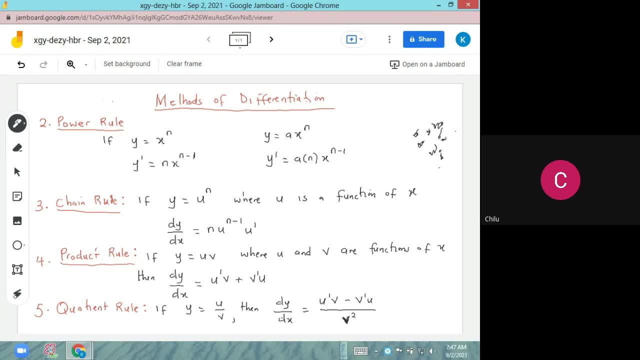 the deriv, the derivative. We find the derivative of u because we are saying u is a function of x. It's not like x, It is a function of x, like two x squared plus four. 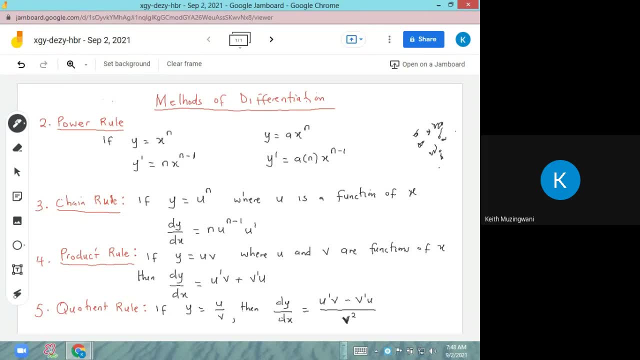 That is u, to the power seven, That is n. So you'll see, when we do examples, what we mean by u being a function of x and then differentiating by treating the power first. 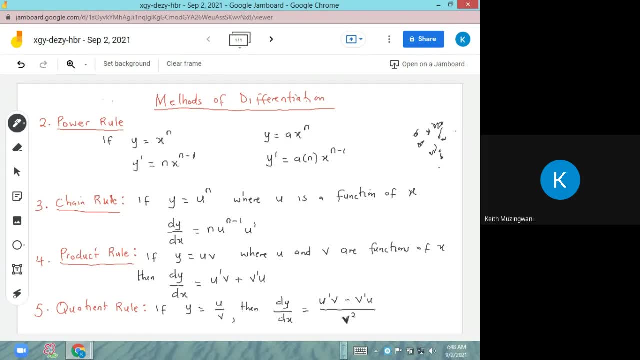 and then the function which is u. Sir, on the power rule there, on the y prime, why are we only differentiating x? What about a? Why are we not differentiating? It's a constant. 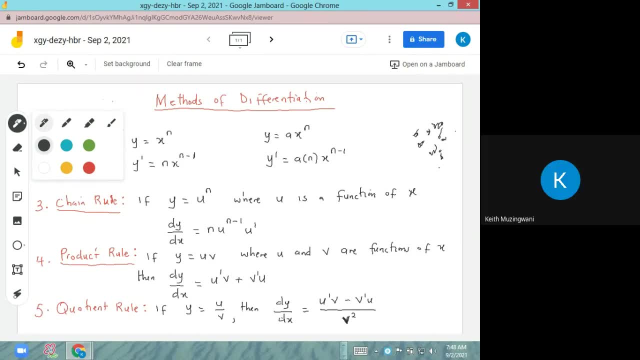 It's just a coefficient to that. So if you try to use product rule, other piece will be zero. So if you try to use product rule, other piece will be zero. Remember that we did. 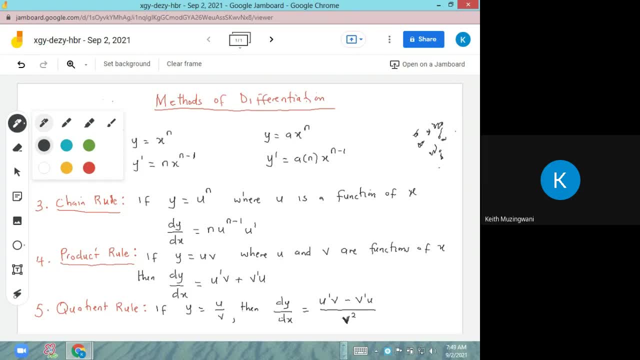 we differentiated the constant using first principle and we got that its derivative was zero. is it Yes, Yeah, So if you take that as the product and then differentiate the two pieces using product rule, 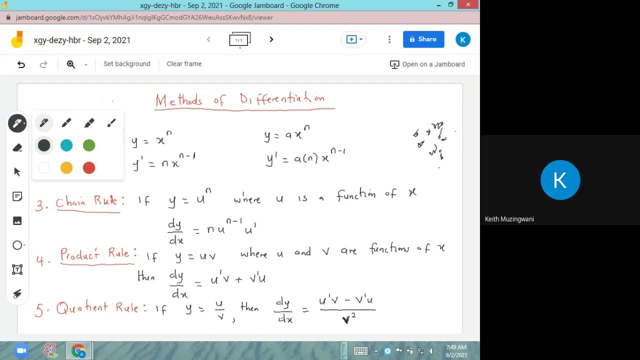 you still arrive at the very thing. zero multiplied by x to the power n will still give you zero, So you rely on a multiplied by the derivative of x to the power n. Okay, I get it. 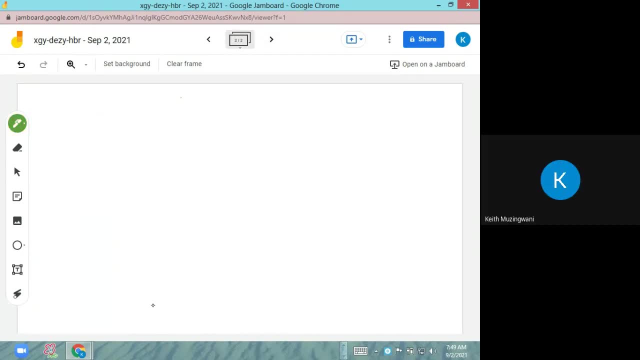 So let's bring a set of examples. Find the y, the x and the y, which is: y is equal to four, b, y is equal to five, x to the power seven minus. 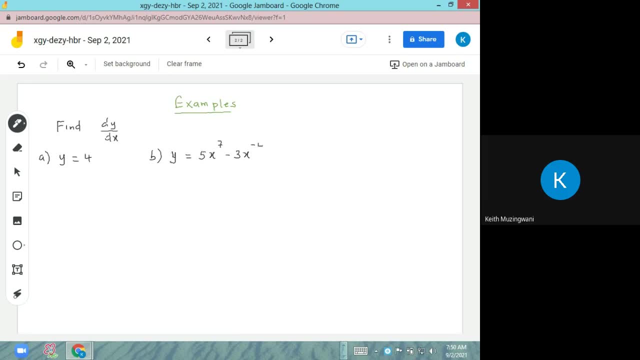 three x to the power negative, four plus plus ten x minus seven. So let's do these two. We'll call this question one. The derivative of of the constant is zero, Because when remember that? 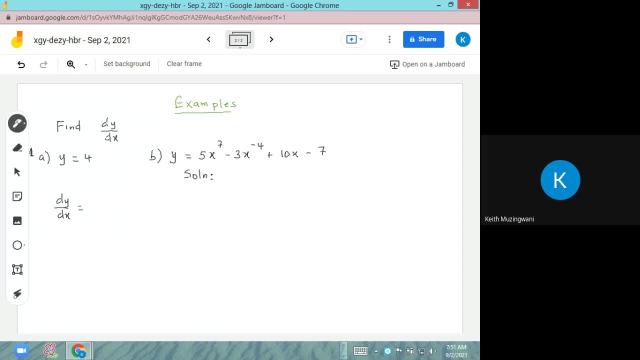 when you are doing binomials, we said this number here can also be written as four: x to the power zero. So if you use the power rule, you have four multiplied by zero, x to the power zero. 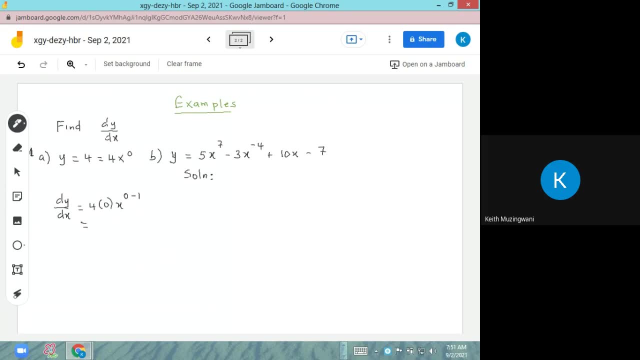 minus one, So get four times zero is zero. That's how we get that derivative there. And then for b divide the x, as usual: five multiplied by zero, plus, plus, plus plus. 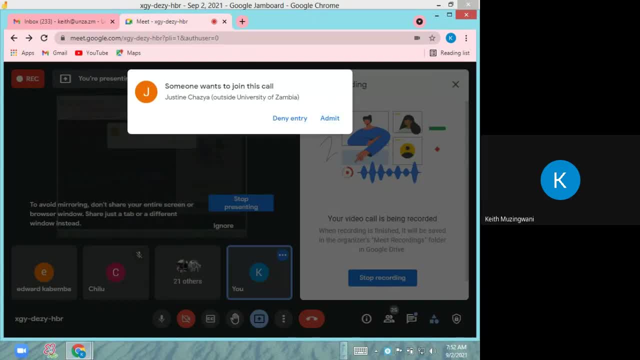 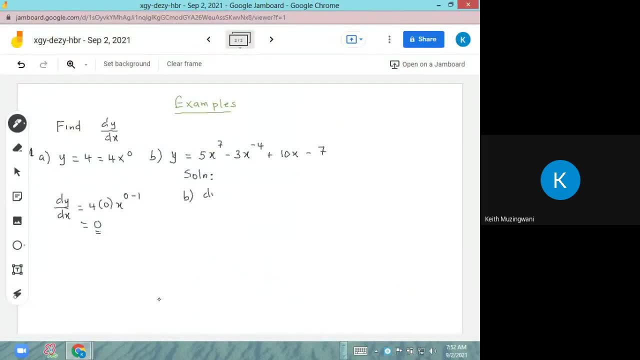 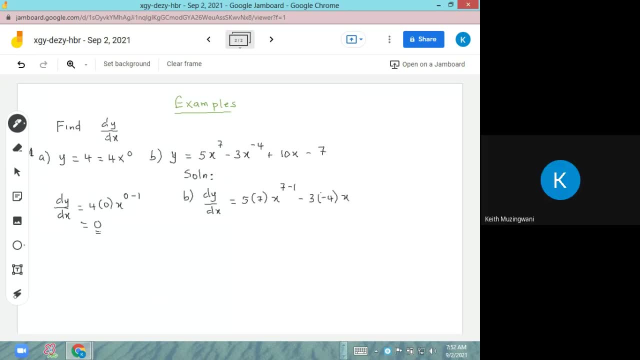 minus three, multiplied by negative four, So x. Please can you take it back to the previous page? This is when i've just joined. This is the page very important. thank you, sir. so X to the power. negative 4 minus 1 plus 10: 1. X to. 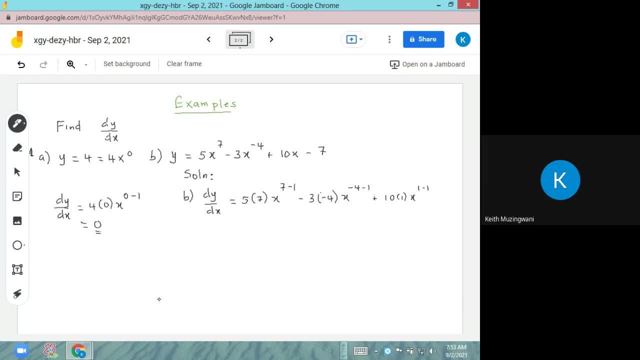 the power 1 minus 1 and then minus 0 derivative of 7, 5 times 7, we get 35 X to the power 6. this becomes plus 12 X to the power negative 5 and plus 10 X to the power 0 is just 1, so we just get 10 there. that's how we find the derivative we. 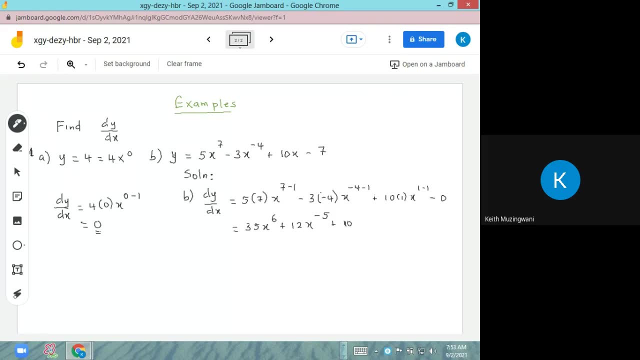 have used power root throughout C. Y is equal to X plus 4 over X. differentiate it. so we are saying we can write this function as X plus 4, X to the power negative 1 because x is in the denominator and it is to the power 1 when we take it up it. 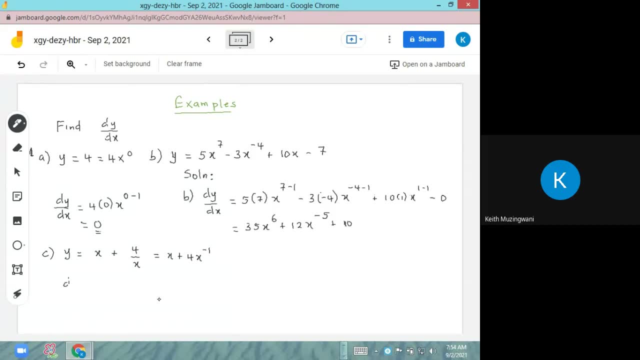 will go up with a negative power, and then dy dx is the same as 1 minus 4 x negative 1 minus 1. so we're getting 1 minus 4 X to the power, negative 2. this is 1 minus 4 over x squared. 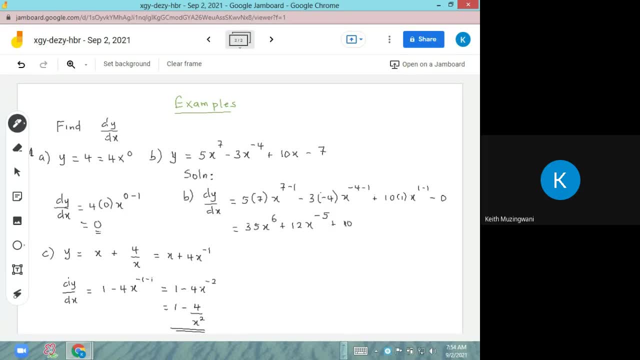 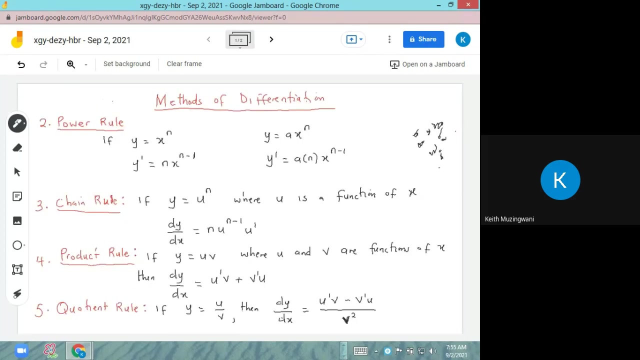 you can still take back the two in the denominator and it will go there as a positive power of x. so example number one, trying to explain what the power rule means, we do. example number two: find f, prime of x. a f of x is equal to 3x to the power 3 minus 4x squared. so how did 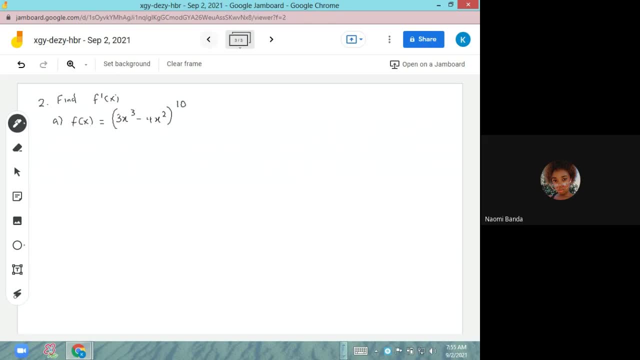 how did the sign change from positive to negative? on question c, from x plus one, oh x plus 4x when so, so it became this: is it? yes? then when differentiating the derivative of x is just one, then the derivative of four, x to the power negative one, we drop the power. 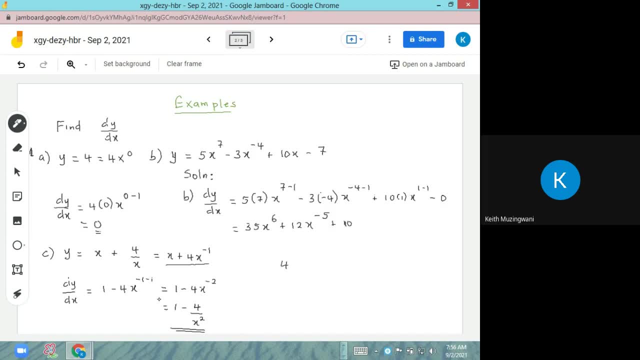 so we'll have. we'll have four multiplied by negative one, x to the power, negative one minus one, and then there's a one here. so this turns out to be one minus four, x to the power, negative two, which i've written as as this. is it okay? 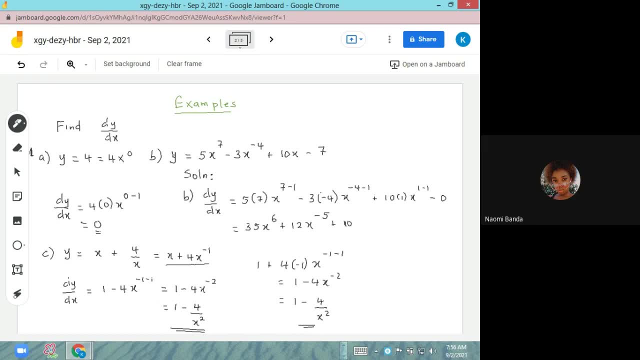 yes, so thank you. okay. so this is a b um f of x is equal to negative. x to the power seven. maybe we put something else: negative x to the power one over three plus four. x to the power negative half. everything in the square root, we differentiate. 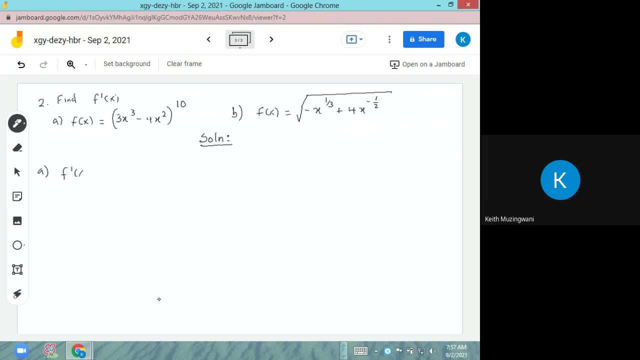 for a f prime of x is going to be: or we can do it slowly- we let u to be 3x to the power 3 minus 4 x squared and then differentiate u. we'll get 9x squared minus 8 x. from there we'll go back to f and write f as u to the power 10. we understand that it's a derivative. 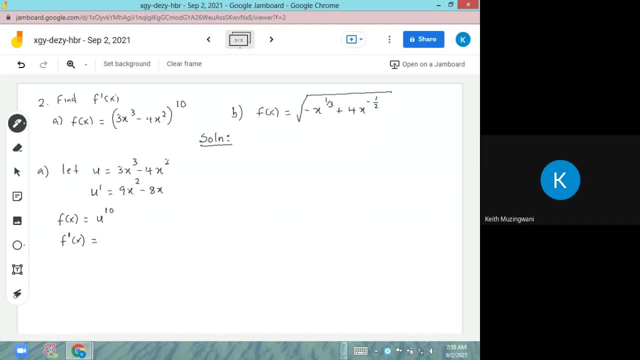 is going to be 10, u 10 minus 1 multiplied by u prime, because we know u is a function of x. that's what the chain rule says. then now we substitute what u is, so we have 10. u is 3x to the power, 3 minus 4x squared. 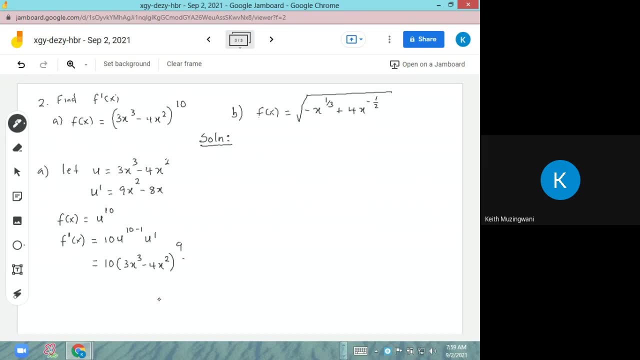 10 minus 1 is 9, and then multiplied by u prime, 9x squared minus 8x. that's what we meant by u prime, because every part must be touched when you're differentiating, so you differentiate the power. first, keep everything inside the brackets, fixed, and then 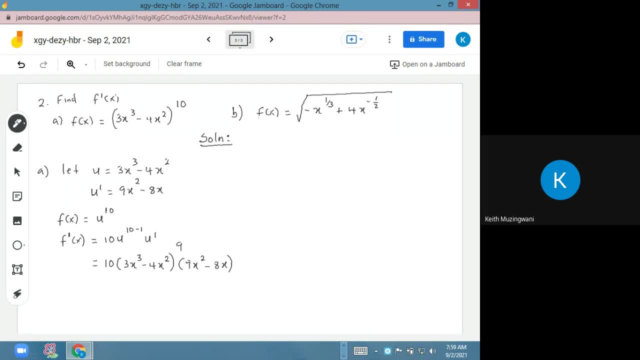 when you're done with the power, go inside the brackets. differentiate everything that is there for b. we can write this function as negative x to the power number three plus four x to the power. negative half to the power half. we know the square root is also half, and then we let u be negative x. 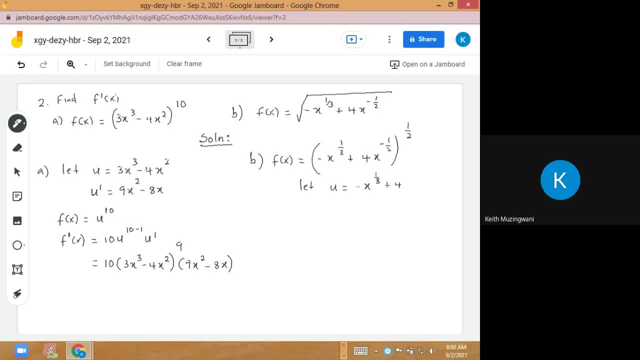 to the power one over three plus four, x to the power, negative one over two, and then differentiate u, we'll get negative one over three x, one over three minus one plus four. negative half x to the power, negative half plus one minus one. we simplify this: we get negative one over three, x to the power, negative two over three minus. 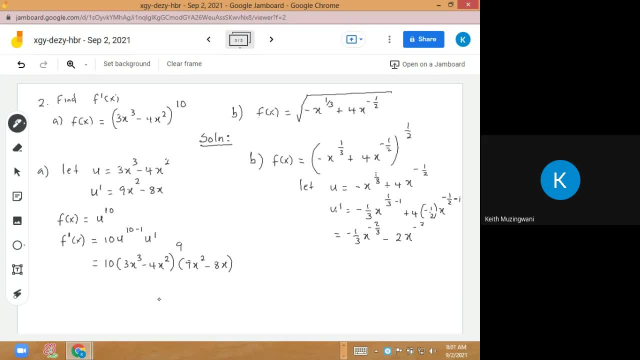 two, x to the power negative three over two, and then we can write f of x as u to the power half, so that it's a derivative, so that it's the derivative and becomes half u to the power half minus one multiplied by u prime, when we substitute: 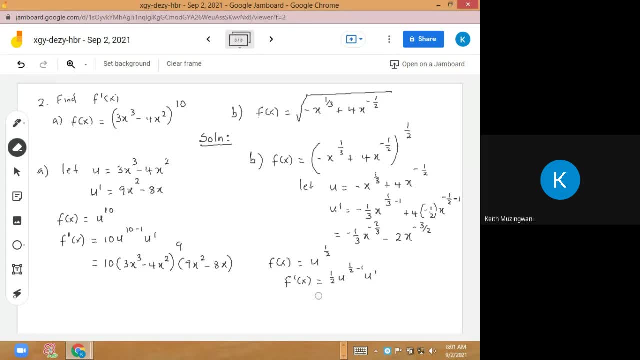 so when we substitute, this is equal to half. u u is negative, x to the power one over three plus four, x to the power, negative, half to the power. half minus one, we get negative half. and then u prime is negative one over three, x to the power, negative two over three. 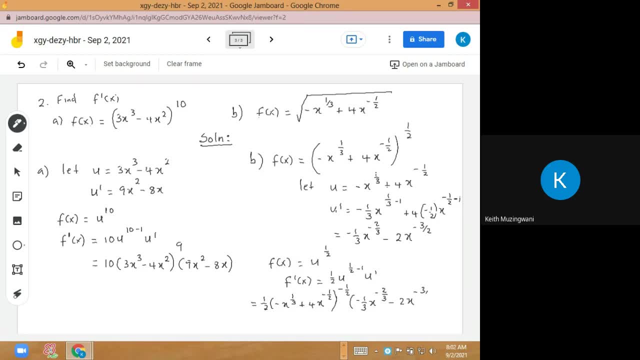 minus two, x to the power, negative three over two, this becomes the derivative of f. this is how we use chain rule. so you make sure that every piece of the function is differentiated. you start with the power. fix what is inside when you are differentiating certain parts. 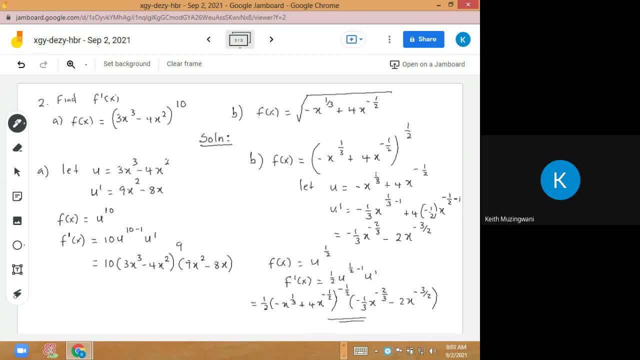 the other parts are differentiating will remain fixed. so when differentiating the power, you leave the function inside as it is. when you're done with the power, you leave the power as it is and differentiate what is inside it. so another example, example three. so another example three: find. 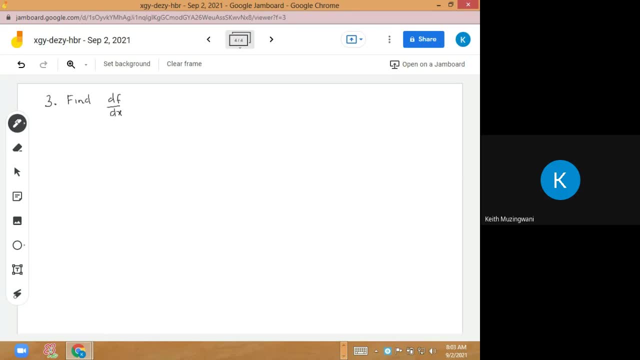 find the f, the x, a f of x is equal to three x squared minus one multiplied by four: x to the power three minus seven x minus seven, x to the power four. so this is a product. if you attempt to start squaring, you need to start expanding a lot of work. 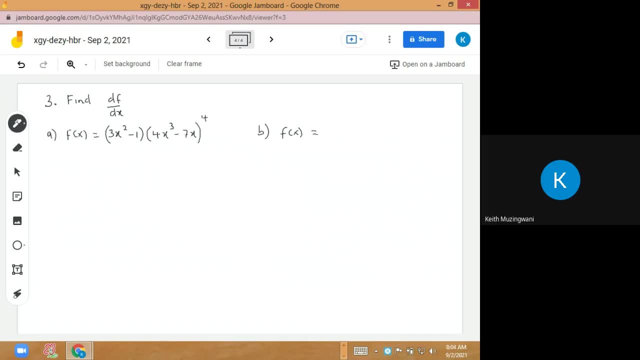 b f of x is equal to the root of x plus one multiplied by one over three. i mean multiplied by b. f of x is equal to the root of x plus one multiplied by one over three. i mean multiplied by one over three. so you can see as we go down step by step. 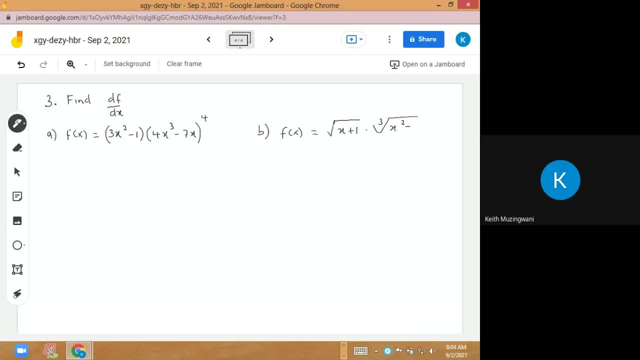 we have a x square minus two minus two, that is the product of x squared solution. we have a that's a product, so directly we let you to be one of them right there. that's where it gets two. in this case, we have a product from from a product from a product. we have a product from a product that's a product and the product. directly, we get u to be one of them. 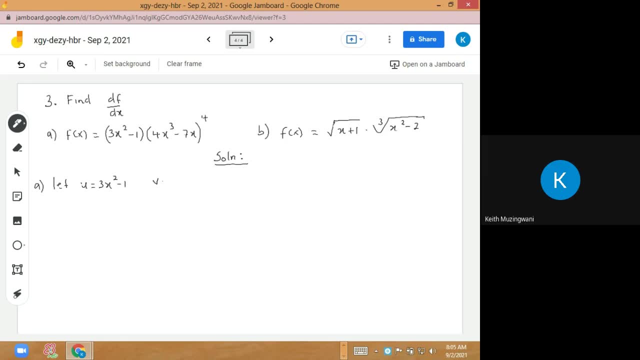 of them, v to be 4x to the power 3 minus 7x, everything to the power 4, and then differentiate u, we'll get 6x. differentiate v, we'll get 4, multiplied by 4x to the power 3 minus 7x. 4 minus 1 is 3, multiplied by, we differentiate now the 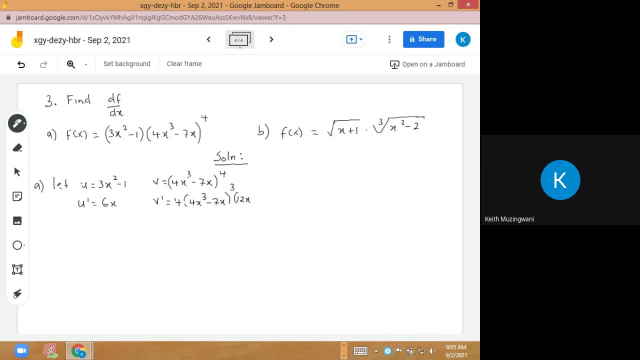 inside of 4x squared minus 7.. Then we are saying the f, the x is equal to u prime v plus v prime u, meaning that u prime is 6x, v is 4x3 minus 7x to the. 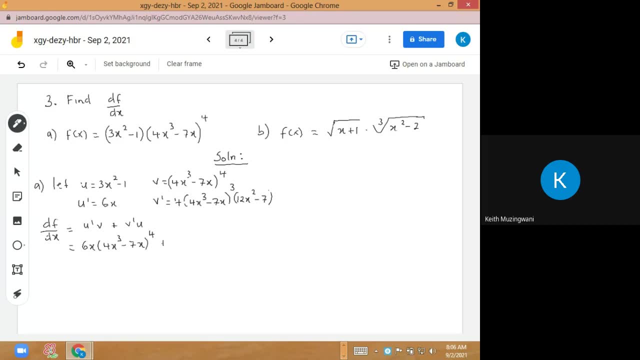 power 4 plus v, prime is 4, 4x3 minus 7x. to the power 3 multiplied by 12x, squared minus 7, multiplied by u, which is 3x squared minus 1.. Then we are done. No much simplification is needed. 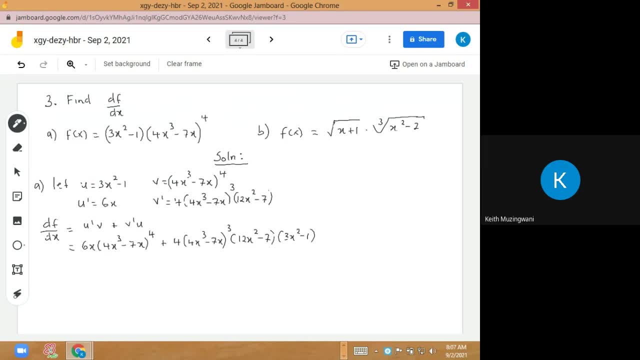 Thank you. When you are taught to differentiate For b, we let u be x plus 1 to the power half, so that its derivative becomes half x plus 1 to the power negative half multiplied by the derivative. The derivative of x is 1.. The derivative of 1 is 0.. 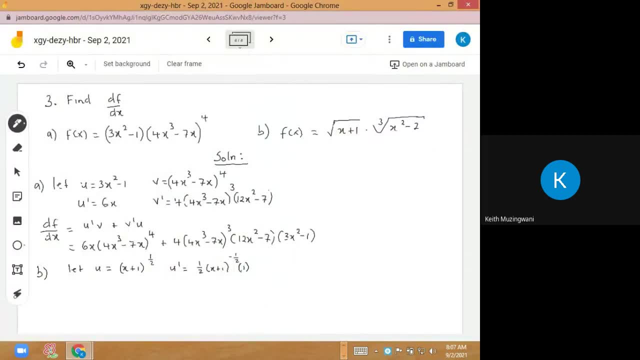 So we get that, and then we let v be x squared minus 2 to the power 1 over 3.. The derivative of v is going to be 1 over 3.. x squared minus 2 to the power negative, 2 over 3 multiplied by 2x. 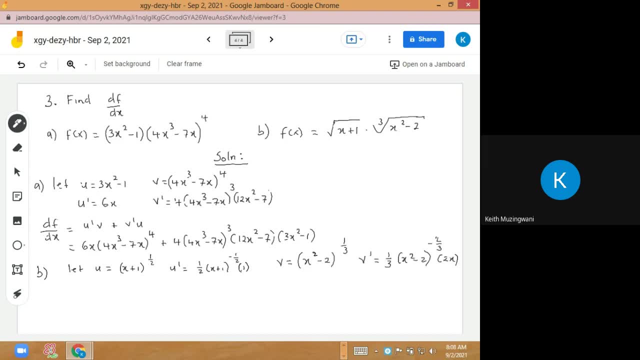 derivative of the inside, and then df, dx is equal to u prime v plus v prime u. this is the same as half x plus 1 to the power negative, half multiplied by v, which is x squared minus 2 to the power 1 over 3 plus v prime. 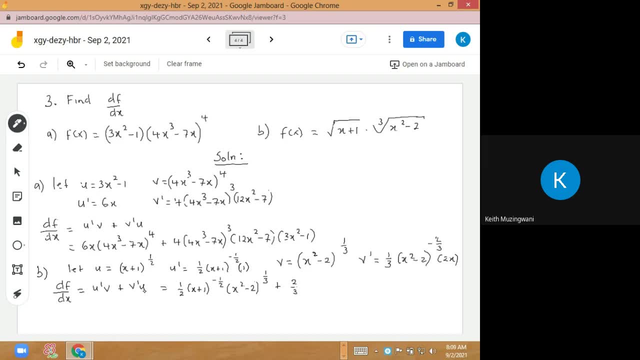 which you can write as: 2 over 3x multiplied by v, multiplied by x, squared minus 2 to the power negative. 2 over 3 multiplied by u and u is x plus 1 to the power half. so this becomes the derivative of f or b using product u. 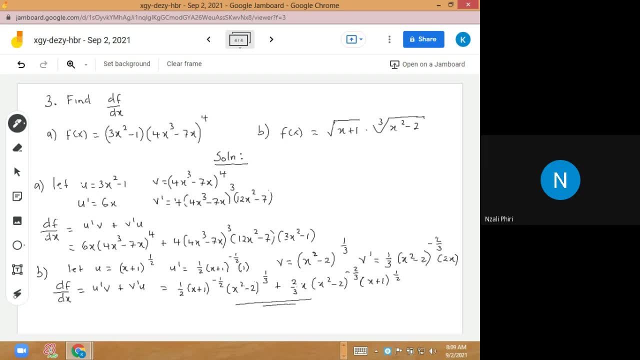 soiosa. so so and the answer, the last part of the answer. i've written 2 over 3. i've written 2 over 3 x. is it not supposed to be one over three? so it's supposed to be one over three button. is this two here? 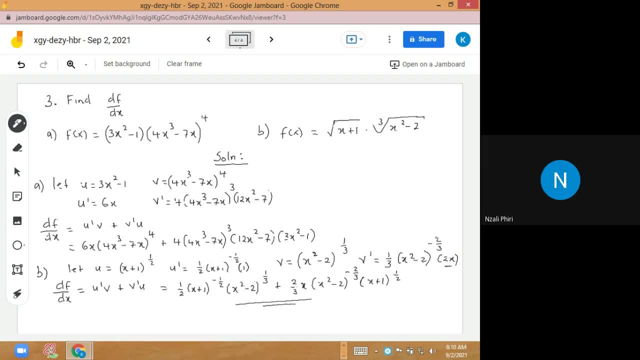 three button is this. two here, sir, on a, when you are finding v prime, your use general. yes, so the, but you have seen that in every rule we have used uh, so these rules will be coming in. so you find yourself doing product rule, using product rule, but in product rule. 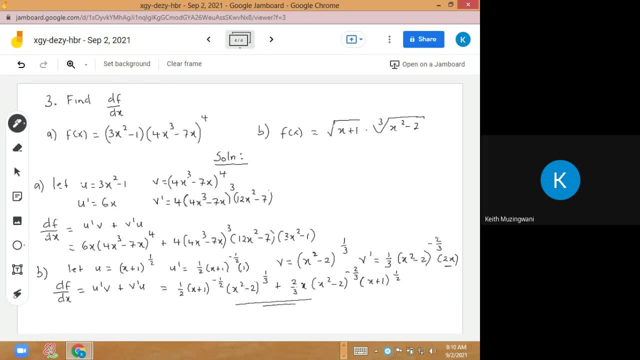 when you're trying to fetch at the pieces you find again they are. they also laying on general, general, the name on our. so the example three, example four: i'm sorry a minute, let me just so he's done. i'm sure, sir, sure sir, okay, i know her. 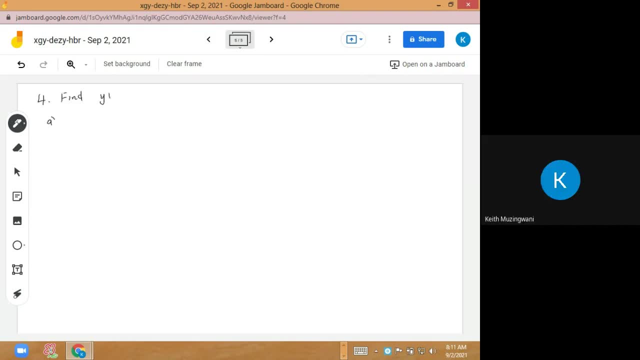 hmm, yeah, so y is equal to 3x plus 1 over x squared minus 10 b, y is equal to a four x squared multiplied by x plus 4. to the power 2 over x. to the power uh, to the power 3 over 2. 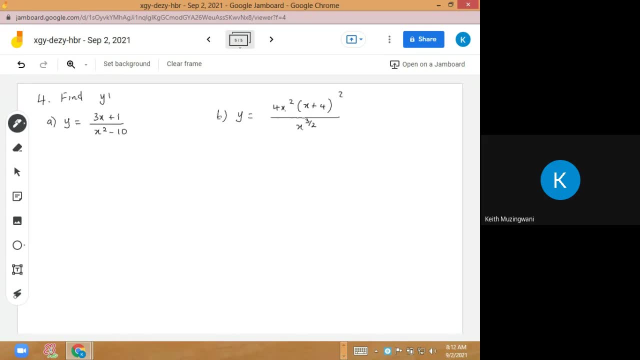 4x squared, multiplied by x plus 4, to the power 2 over x to the power uh. to the power 3 over 2. so that's it for this video. i hope you found it helpful. if you did, please leave a like and subscribe to my channel, and i will see you in the next video. bye, bye. 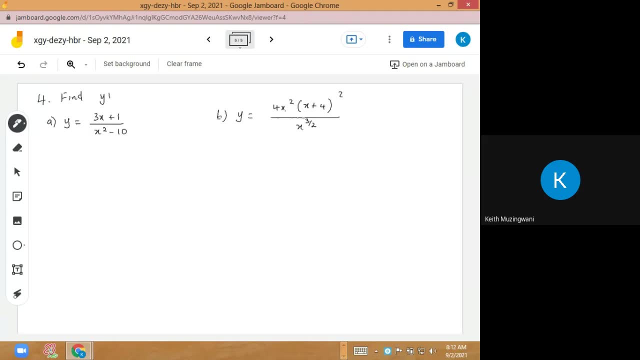 solution for the first one. you can see that's a fraction. so whenever you have a fraction you use quotient true. so you let u be the numerator and v be the unit and then differentiate u to get three. differentiate v will get 2x and then find y prime, which is u prime, v minus. 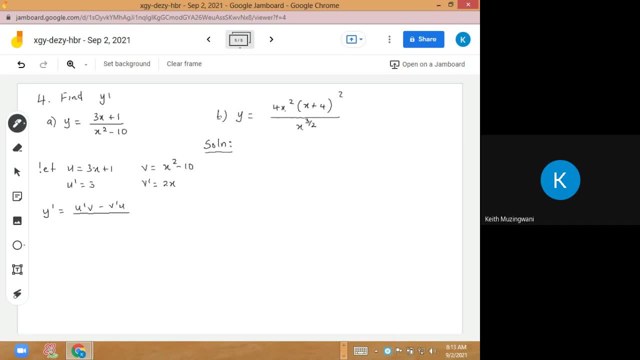 v prime. u over v squared. this is u prime is three v with x squared minus ten minus v, prime is 2x. u is 3x plus 1 over v squared. is x squared minus 10 squared, it looks like it's: this one is nice to simplify. so we have 3x squared minus 13 minus 6x squared minus 2x. 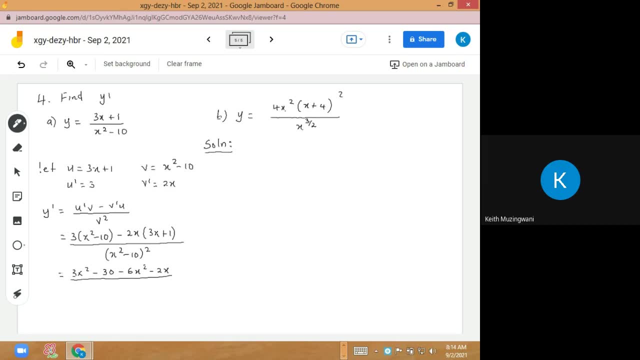 over x squared minus 10 squared, and the other step would be negative: 3x squared minus 2x minus 13. over x squared minus 10 squared, we got to b. so this was a b. let u be 4x squared multiplied by x plus 4. 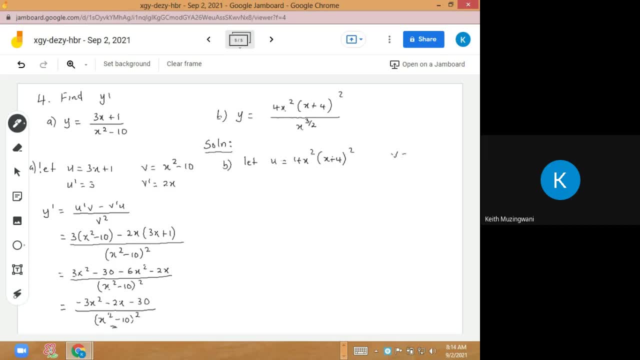 squared and v bx to the power 3 over x. when differentiating u you use product rule. so first differentiate 4x squared, we'll get 8x, then multiply it by x plus 4 squared and then we add: we differentiate 4x, x plus 4 squared, so drop 2, we'll have x plus 4 multiplied by 1, the derivative of x plus 4, and 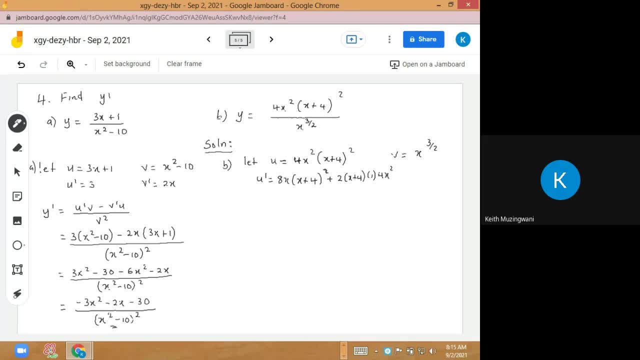 then multiply it by 4x squared. we simplify this. it will be 8x x plus 4 squared plus 2 times 4. we'll get 8x squared and then x plus 4. then we go to v and differentiate v. we drop the power and remain with x, 3 over 2 minus. 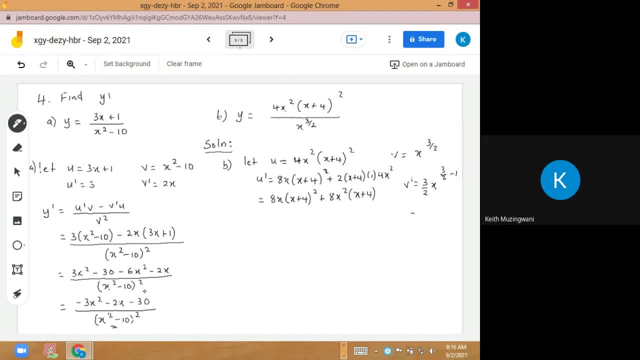 1 um. this is the same as 3 over 2, x to the power, 1 over 2, and then we have y prime. then y prime is going to be u prime by minus v prime. u over v squared, that is f x squared over u prime is 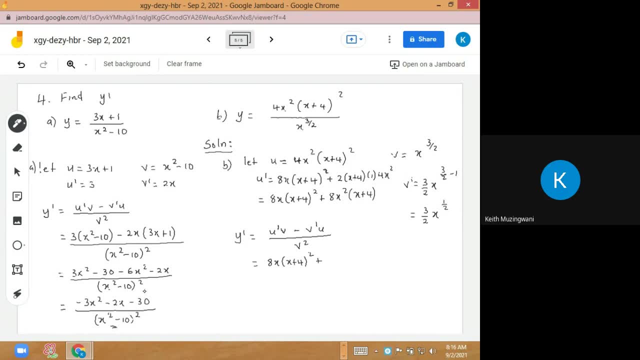 4 squared plus 8x squared x plus 4. this whole thing is: u prime multiplied by v, which is x, to the power 3 over 2 minus v. prime 3 over 2, x to the power half multiplied by u, which is 4x. 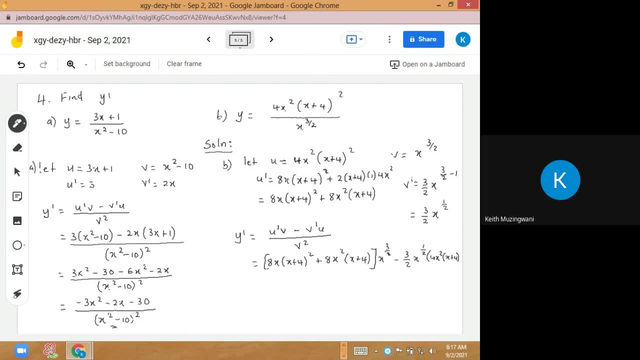 squared, x plus 4 squared, and then we close everything over v squared to just come out as x to the power 3. since we multiplied by x to the power 3, we get x to the power 3, x to the power 3 x 3 over 2. when you square this, these two will cancel. you have x to the power 3, so we have this. 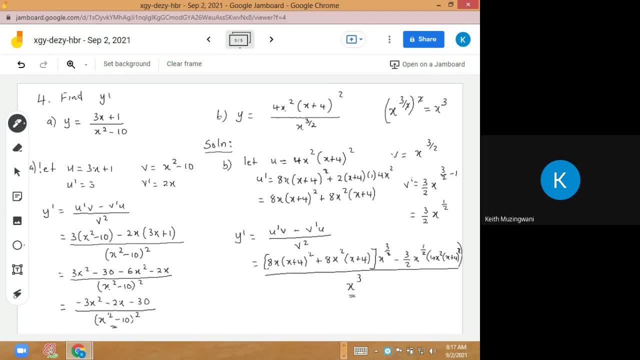 as y prime. we have used quotient rule, so this means it's more likely to change it like. i'll give an example. first example: here's quota: 3x plus 1, then over x squared minus 10. but we'll change it in the form of: 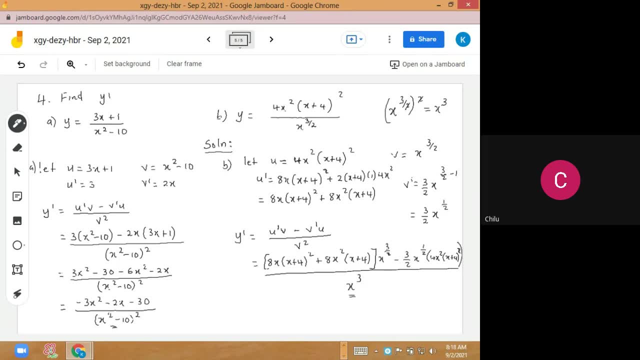 in the form of product, we did work, or who is over the graph, you know for imperative it can work, but the difference is the same. so is it that wherever chain rule is involved, you have to use the other rule before tenure, like how product rule was used before the tenure? 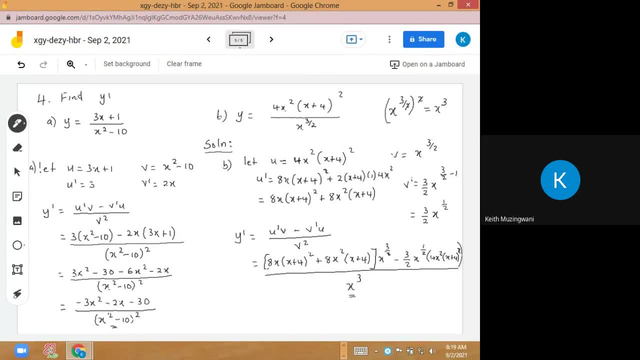 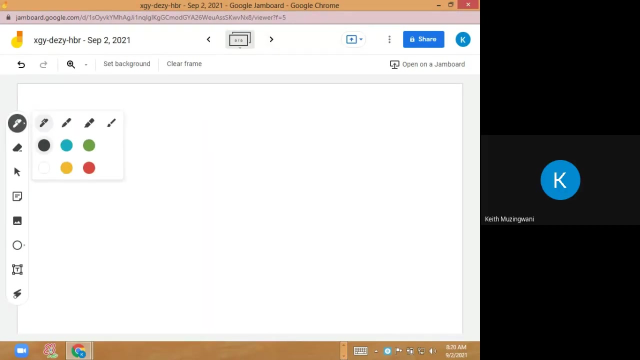 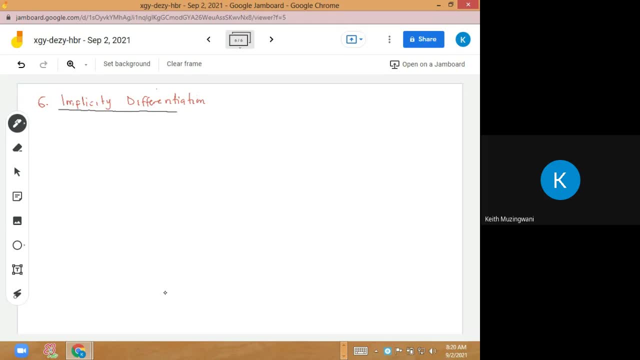 Okay, this one, if you observed in the previous rows, when you have y is equal to 4x squared, for example, and we are asked to find y prime. Now y prime is the same as dy dx. Okay, so what we do here is for you to move from this step to y prime. 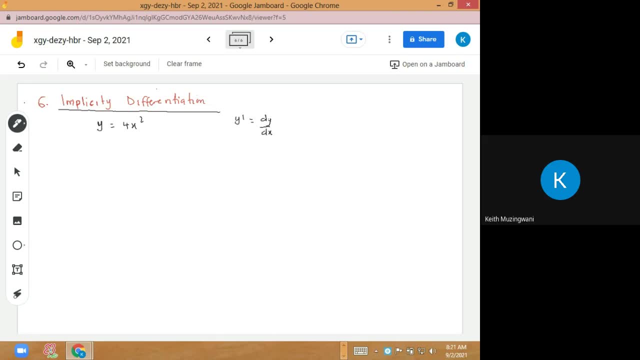 you actually differentiate y as if it was x. When we say the derivative of x, we get 1.. So when we say dy dx, you first differentiate y, you get 1, and then you multiply by dy dx Because you have differentiated y with respect to itself. 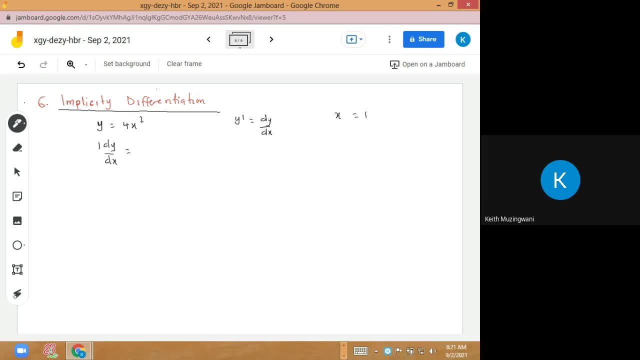 when you actually are supposed to differentiate with respect to x. And then on the right, you differentiate x, 4x squared with respect to x, so you get 8x, But 1 times dy dx still remains dy dx, which is 8x. 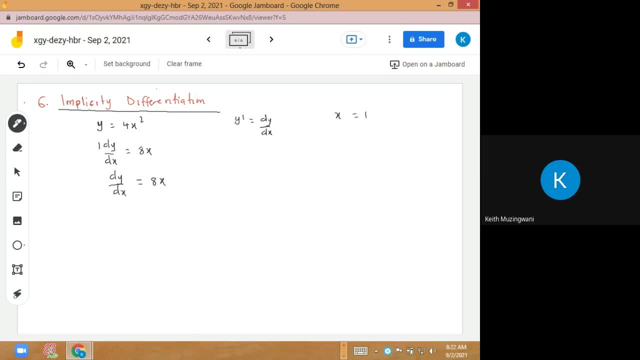 Now the point here is that you can still do this even if y was squared. Suppose you had y squared. It's equal to 8x, So you have 4x squared. Instead of solving for y, you could just differentiate y squared. 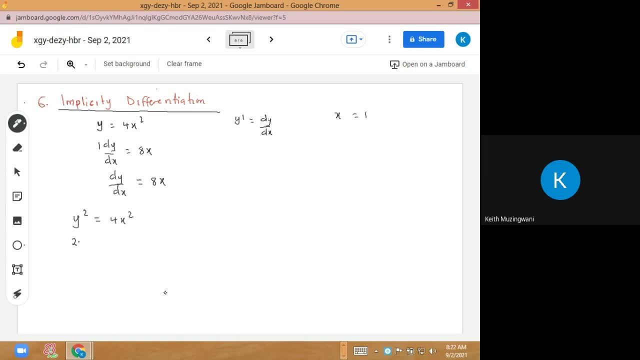 as if you are differentiating x squared. So you say 2y, But because you have differentiated y squared, as if you are doing it with respect to y, you multiply it by dy, dx and then differentiate 4x squared with respect to x. 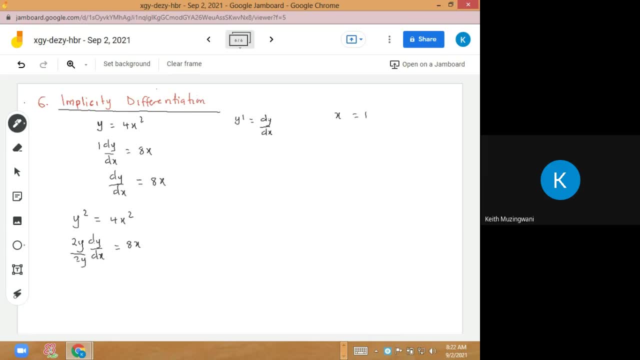 you get 8x, So you divide by 2.. You divide by 2y. So your function is: Your function is going to be: dy. dx is equal to 8x over 2y. So this method where you don't bother yourself to solve for y, 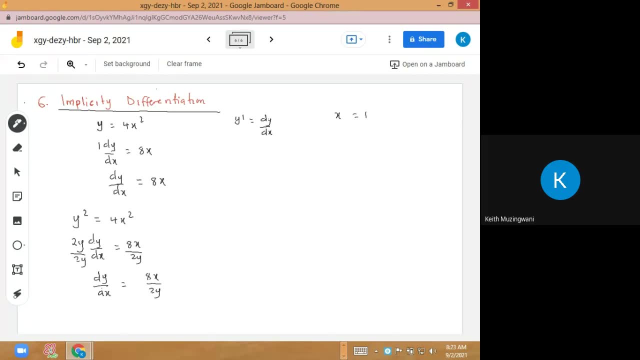 you just differentiate y wherever it is and just remember to multiply by dy dx every time. you differentiate y is what we call implicit differentiation. It doesn't have a formal way of writing it. That's why we write this Here For it, if we are to force it to be formal. 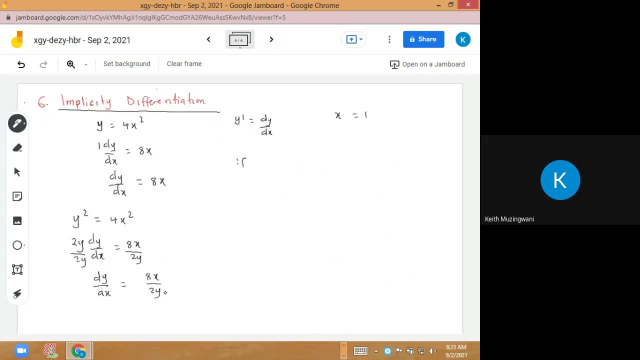 we'll just say: if you have a situation where you have y to the power, n is equal to some function of x, then you would say: to find dy dx, you would say you have ny n minus 1, dy dx is equal to f prime of x. 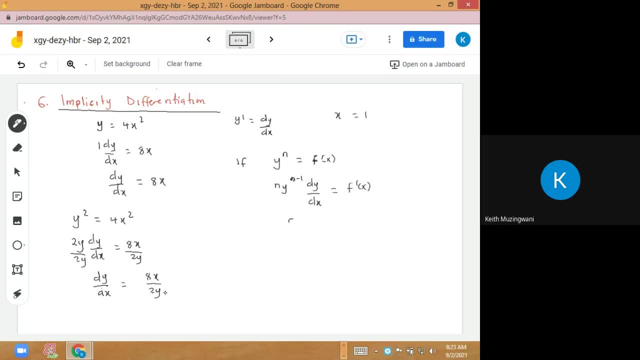 And then leave dy dx alone, equal to f prime of x divided by ny n minus 1.. Yeah, Or have such a thing If we force it to be formal, Excuse me sir. Yeah, Can you repeat the explanation on just starting from y squared is equal to 4x squared. 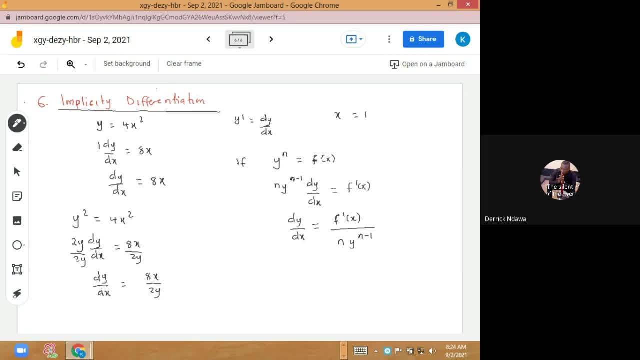 How to let dy dx be the subject. So the first thing you do is you treat y squared as if it is x squared and use power rule on it. So differentiate y squared using power rule, it's going to be 2y. 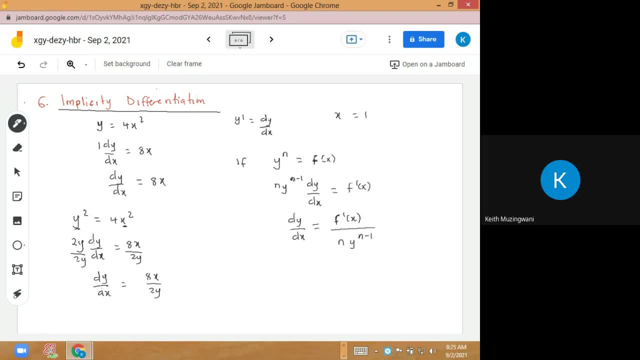 But y is a function of x, so you multiply it by dy dx And then differentiate for x squared with respect to x, so you have 8x, And then you are solving for dy dx, So you divide throughout by 2y. 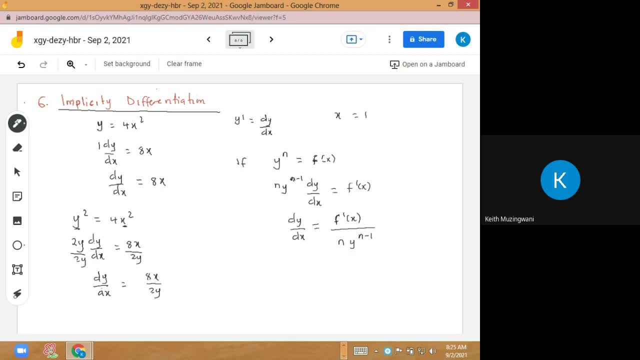 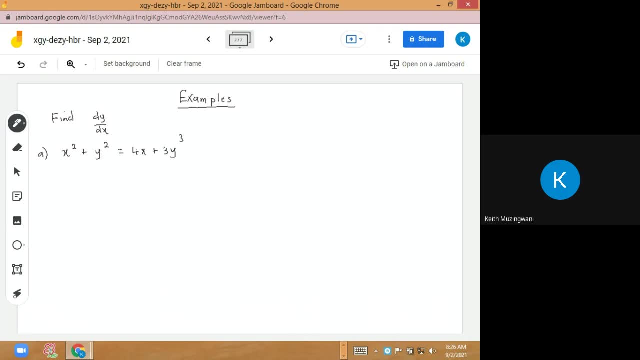 5y and be negative. x squared plus y squared is equal to 1 solution. so say: okay, this is not a difficult thing, instead of us trying to solve for y, which may be so difficult, if not impossible, manner. so say, okay, this is just the same as. 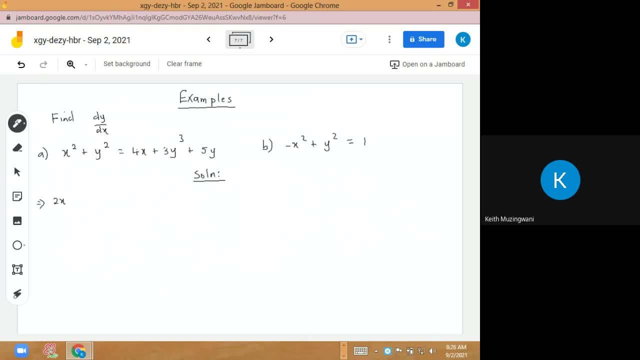 differentiating x squared will get to x. differentiating y squared will get to y. but because it is y, we multiply by dy. dx is equal to differentiate 4x, we get 4. plus differentiate 3y to the power 3, we get 9. 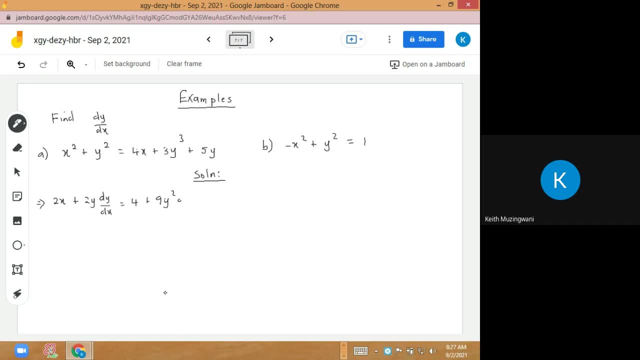 y squared, but because it is y multiplied by dy dx plus differentiate 5y, you get 5. but because there was a y, you put dy dx and then you are solving for dy dx. so you put together all the dy dx, anything that has dy dx. 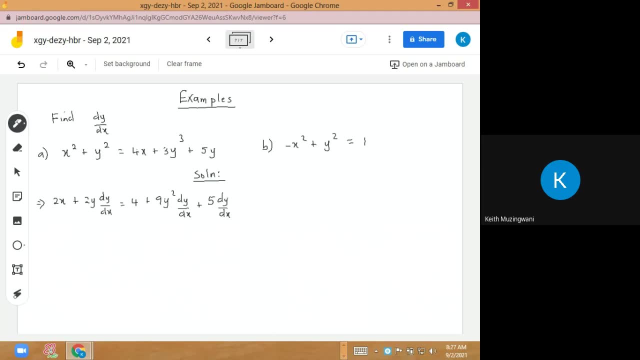 you correct them and put them one side and every everything else you take the other side. so this implies that you have 2y dy dx minus 9y, squared dy dx minus 5 dy dx is equal to 4 minus 2x. and then fact out dy dx. 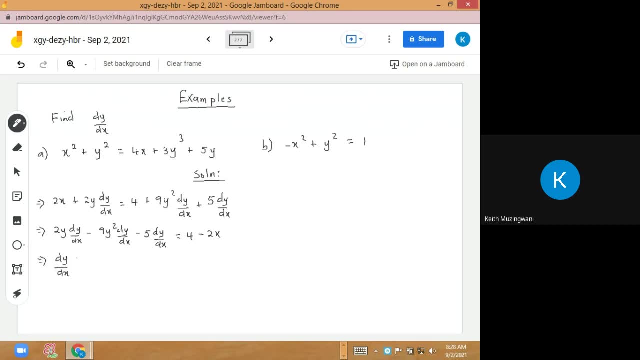 you get: 2y minus 9y squared minus 5 is equal to 4 minus 2x. this means that dy dx is equal to 4 minus 2 x divided by 4y minus 9x and minus 9y Minus 9y squared minus 5.. 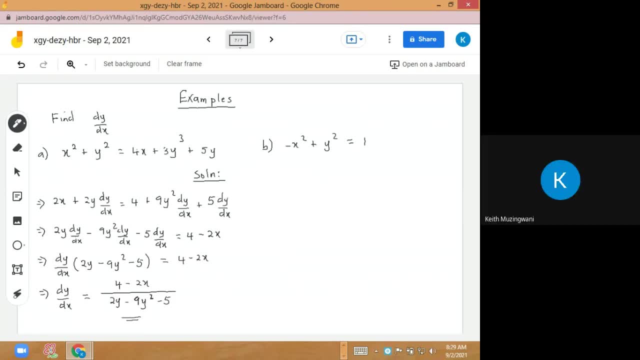 Quasi da. Yeah, quasi da. So that's how you do the derivatives here. So this was A. Let's go to B. You differentiate negative x squared, so you have negative 2x, Plus differentiate y squared, you have 2y. 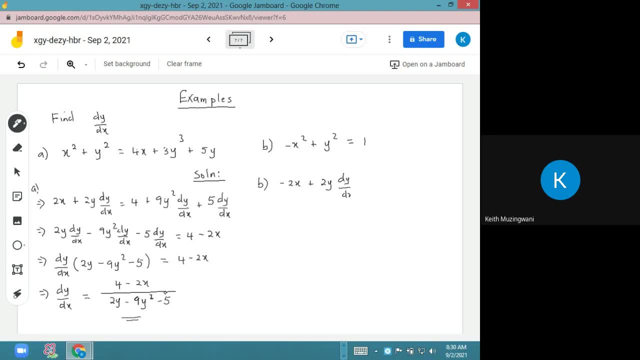 But because it is y, you multiply by dy, dx is equal to 0.. This means that we have 2y. dy dx is equal to positive 2x. Divide by 2y and divide by 2y. 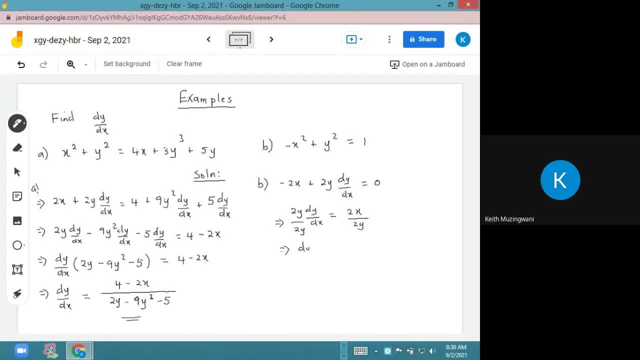 so you get dy dx to be equal to 2x. So that means x over 2y, which is equal x over 4y. We got x, which is equal to x. Where's the negative one? Oh, we took the other side off. 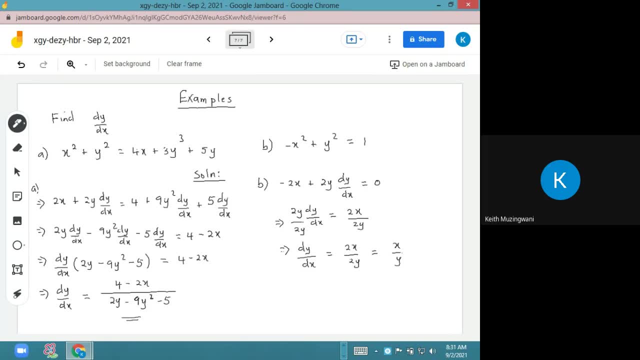 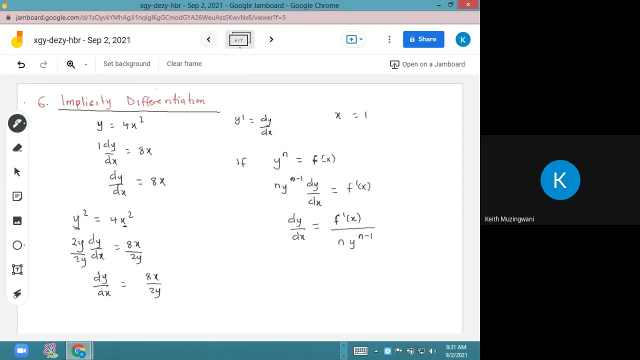 All right, Sorry, Yeah, so this is what we call differentiation. so in here: calculus, derivatives- these are the only six methods that exist on. derivatives is an example on impressive, yeah, bring it up open bracket X minus Y close to the powerful. mm-hmm, it's a good: X plus Y plus 5, so solution. 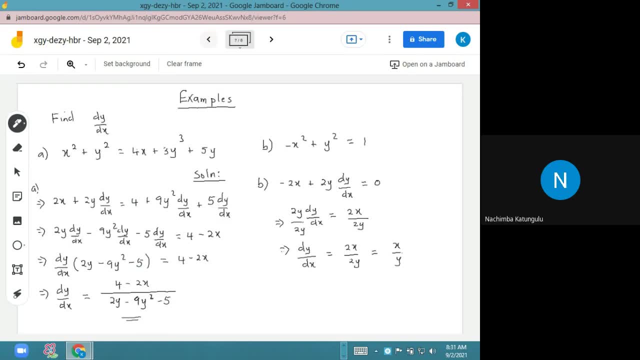 mm-hmm, I can't repeat the previous page. you want you, I have. thank you, okay. so here we use, here we use general for this piece. we first drop, therefore, and keep everything else inside. 4 minus 1, we get 3 multiplied by the derivative of the inside derivative of X is: 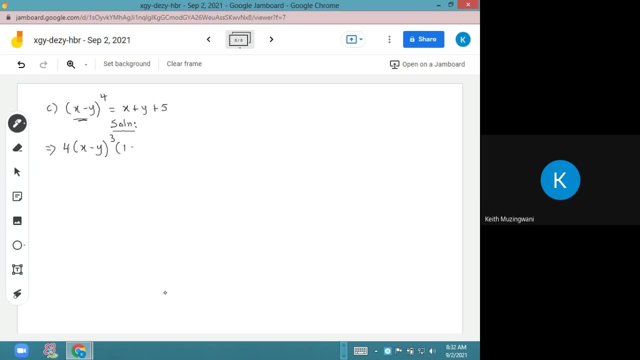 1. derivative of negative Y is negative 1, but because it is Y, we multiply by dy the X is equal to. derivative of X is 1. derivative of Y is 1, but because it is Y multiplied by dy the X. so let's, let's be muted. 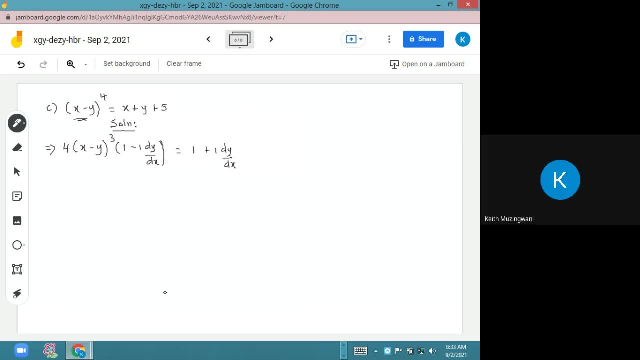 good, then we expand now in expansion. you don't need to break this, just want to break this here. so we'll have 4 X minus Y to the power 3 multiplied by 1, we'll get 4 X minus Y to the power 3 minus. for X minus Y dy, the X which is equal to 1. 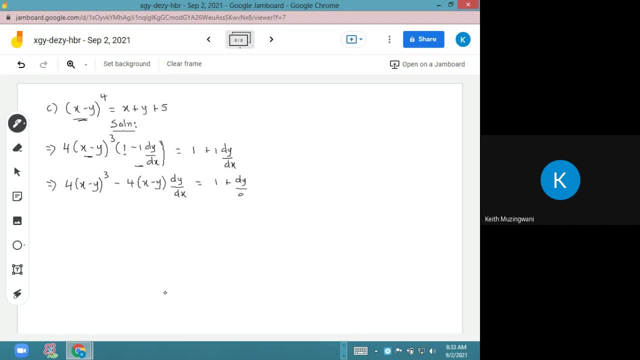 plus the y dx, and then we take this Kover sites. in this one on a side was looking for u IDX, so now let's add to y, to the X, which is equal to one, plus dy dx, and then we take this guy on the other. in this one there are sites because they're looking for dy dx, so that's one right. because we're looking for dy dx and then we take this guy y aside and we're looking for you ID X, select 4, X minus y to the power 3 minus 4 dx plus y dx and w plus string X, and then we take this guy on the other накupal and bearing and b- three elements are here and n plus a primary spaces, Prosex and forixoom logarithmic authority character. this is that, if you're watching, if you don't like. this is confusing and unfortunately 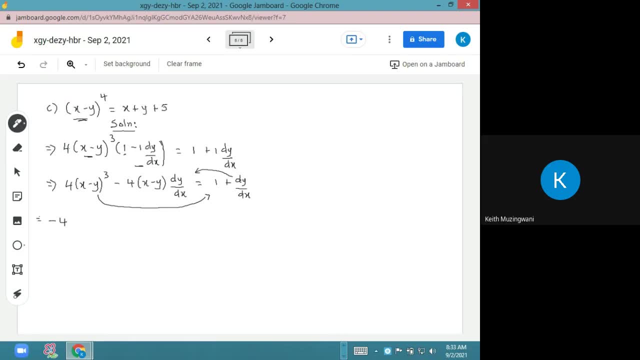 So we have negative 4x minus y dy dx minus dy dx is equal to 1 minus 4x minus y to the power 3.. And then we factor dy dx, then we have negative 4x minus y minus 1 is equal to 1 minus 4x minus y to the power 3.. 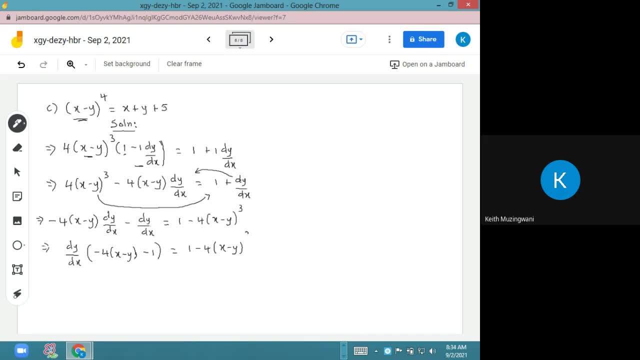 So we have negative 4x minus y to the power 3 and then divide by everything we remain with dy, dx is equal to 1 minus 4x minus y to the power 3 over negative 4x minus y minus 1.. 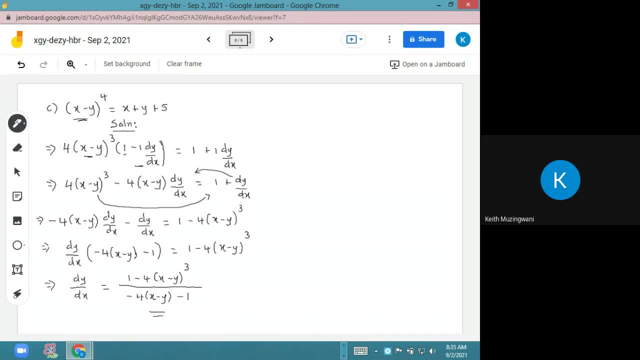 So this is the derivative. The thing of factoring out the negatives on the right is having time. If you have time, you do that, But if it's your first question, you should always know that we're just starting and we have so many things to do. 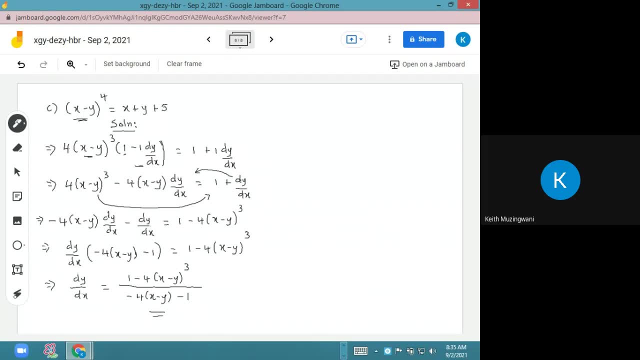 So if you leave it there, you lose no mark. Okay, that is first On the second step. where is the negative 4 coming from? Where is the negative 4 coming from On the second step? So we expand it. 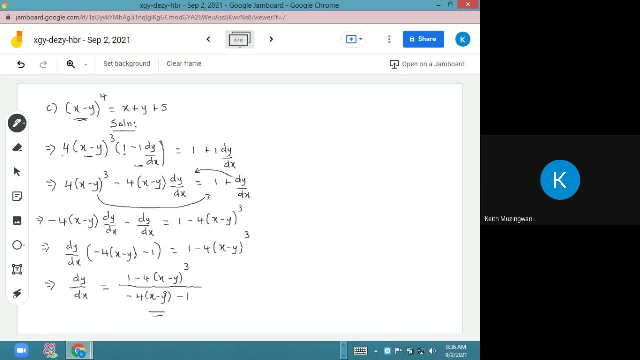 So here we're expanding, We are multiplying this whole thing by 1.. We got this Again, this whole thing by negative, Negative, Negative, 1, dy, dx. So the negative multiplied by positive 4, we get negative 4.. 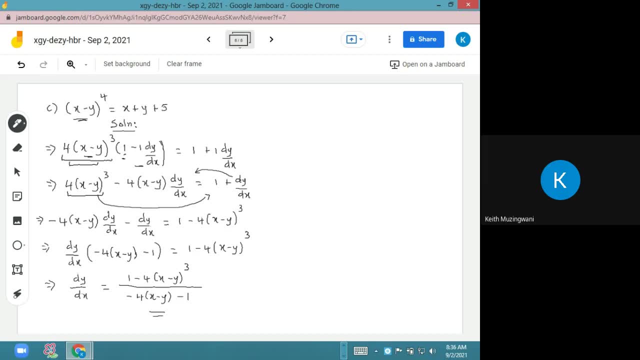 And then everything else follows. So can you explain again, Okay, Okay, Let me pick that question from. Let me stop from talking there, So that I answer two at a time. Okay, So I take negative 1 by Now, when it's negative 1.. 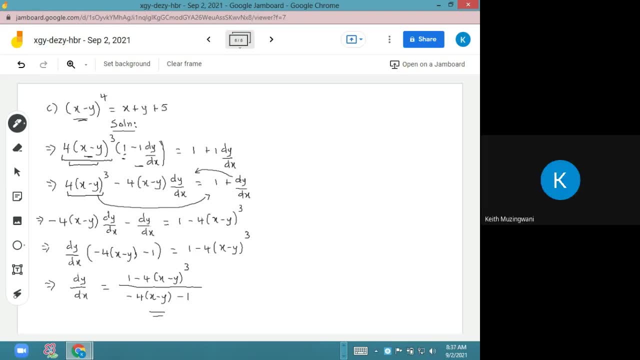 Go ahead, I will Uh-huh. So what I usually do is let me take half. I see that. I find that that feels like negative 1, then negative 2, and it feels negative 4.. I see that informação comes continuously several times. 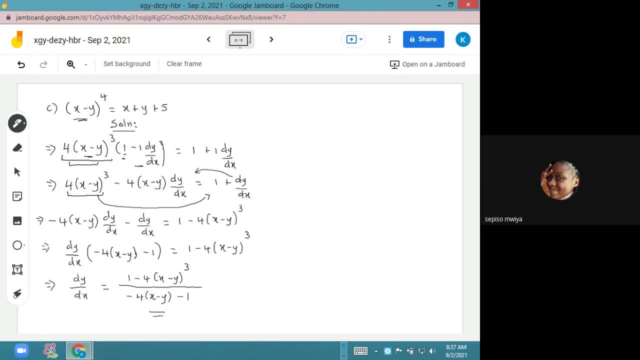 Okay, Okay, Go ahead. Thank you. like we don't. we like not touching x minus with two, x minus y to the power three, but then just expanding for- and this one here is to the power three, this is to the power three. where is it? 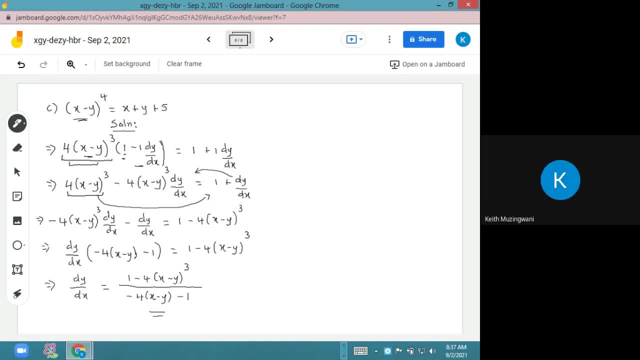 not three, it's four, sir. to the powerful, uh, to the battery wasn't differentiated, we are just differentiating the inside part, instead that we got a great power, sir. uh, we start by touching the power before we go to the info for the power, so you can go back then. 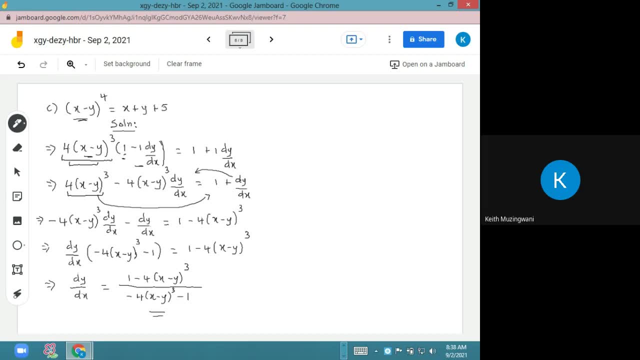 you know what we have is x minus y to the powerful is equal to x plus y plus five, is it? this? here is like u to the powerful. when you differentiate it, you say 4 u3 by u prime, so say 4 x minus y, 3. 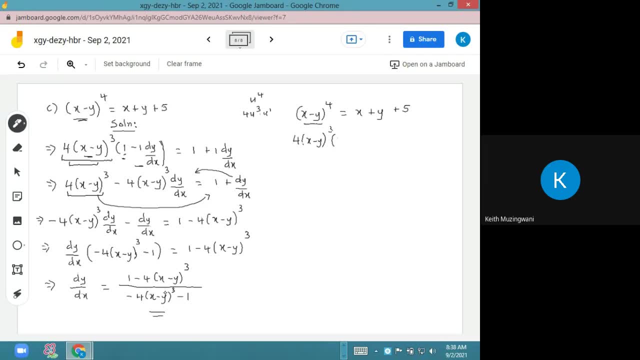 and then u prime. we differentiate x, we get one. we differentiate y, so i have minus 1. multiplied by dy, dx is equal to. we differentiate x, we get one. we differentiate one power, the power. which power? you said to the uh, to the u prime. so ah, it is your prime kind of prime. yes, you confused us. you said you are supposed to put a power. 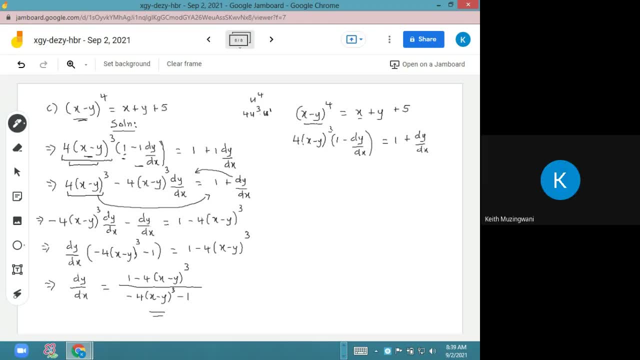 no, look, then here we expand. now. what is this multiplied by one? we'll get four x minus y to the power three minus what is this? multiplied by dy dx, we'll have four x minus y to the power three. dy dx is equal to one plus dy dx. here, here we're just expanding this. 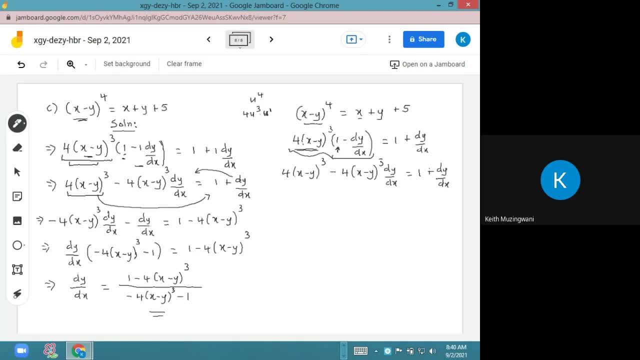 by this: that's all we're doing, okay. and then hello, and then we take this this side and this one the other side, so nothing will change as we take outside. so we have negative four x minus y to the power. three ui dx minus ui dx is equal to one minus four x minus y. 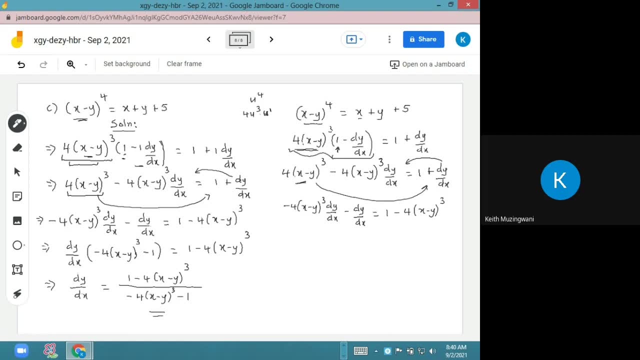 to the power three this one. then we factor out dy. dx will remain with negative four x minus y to the power three minus one is equal to one minus four x minus y to the power three, and then divide by negative four x minus y to the power three minus one, divided by negative four x minus y to the power three minus one. 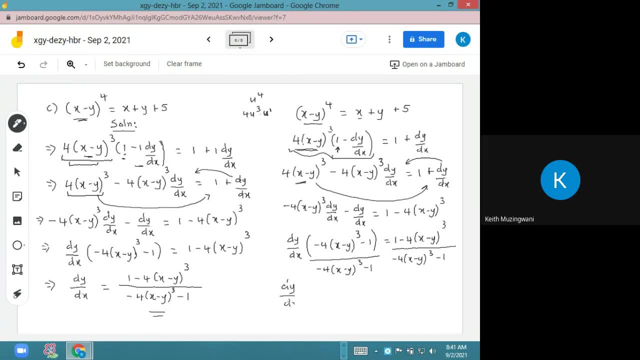 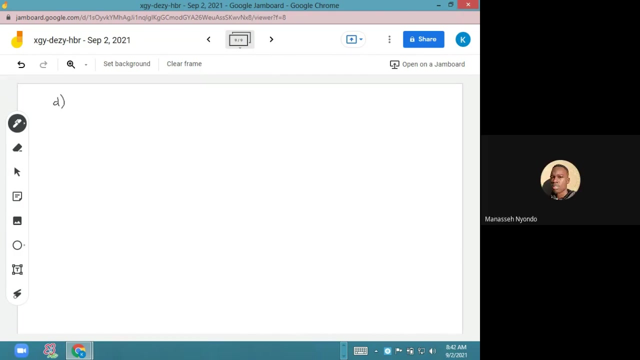 so remaining dy dx is equal to one minus four x minus y to the power three over negative four x minus y to the power three minus one. exactly what we have here. same method, same everything, same method, same method, same n. and then then we're thing that's. 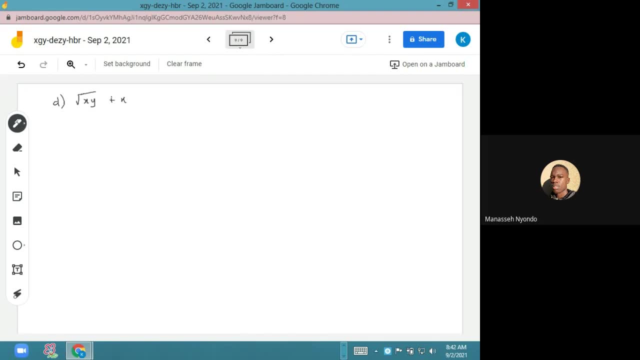 okay, hey, okay, okay, good, yeah. so it goes to zero. the derivative of the constant is zero. so whether we're differentiating zero or any other constant, we still get zero. then we can write the first part as x to the power half, differentiate it as half, x, y, half minus one is negative half, and then this we differentiate as product. 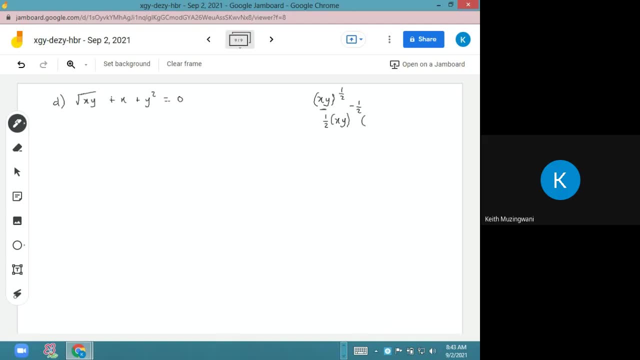 so in case differentiate x, we get one. so we have one times y, which is one plus. we differentiate now with respect to y, so we have x, but because it is y, we have y, dx. so we'll get this represent the first part here, so we have half negative. 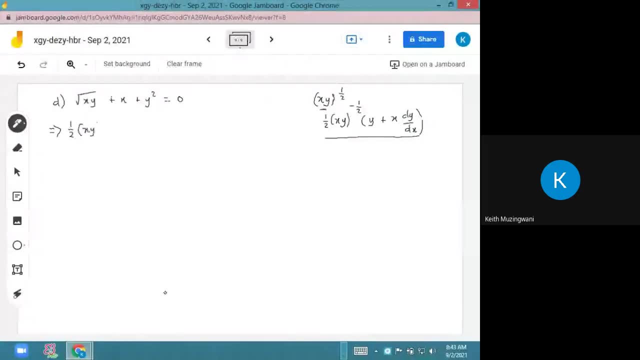 we'll have half x, y to the power negative, half multiplied by y plus x, dy dx. plus we differentiate x, we'll get one. plus we differentiate y squared, we get two y. but because it is y, dy dx is going to give us zero. then we fact out. uh, before we fact out the y dx, we first expand. 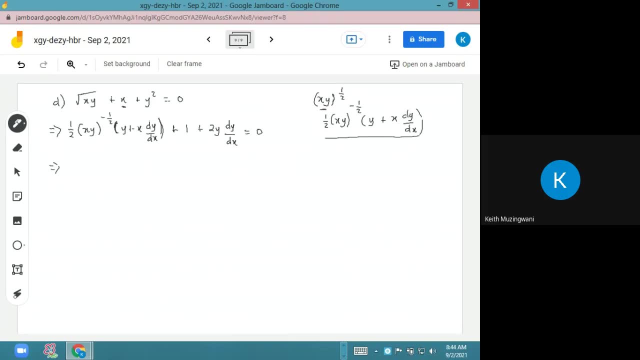 because of these brackets here. so first expand. so we have half x y to the power negative, half half y y plus. let y have plus x over 2 root x, y, x over 2 root x, y x, the y d x, x, the y d x. 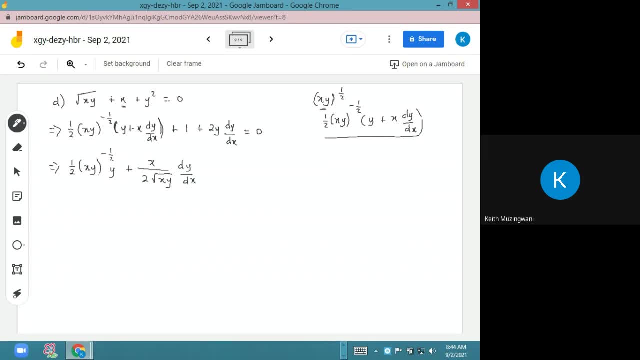 x and then x, and then x plus one plus one plus one plus two, y plus two, y plus two, y, x, dx is equal to zero. so what we're going to do is need to find n equal to x. dx is equal to zero. so what we're going to do is make sure we take that s, x, q. so 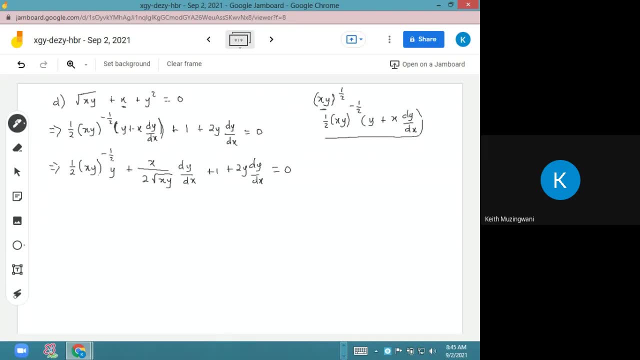 what we have done here is we have written this guy, we've taken it back in the root, but because its half is negative, we've taken it in the denominator. and then this x. here we're multiplying one by this x. that's why we have the x as a numerator. and then we're interested in dy dx. 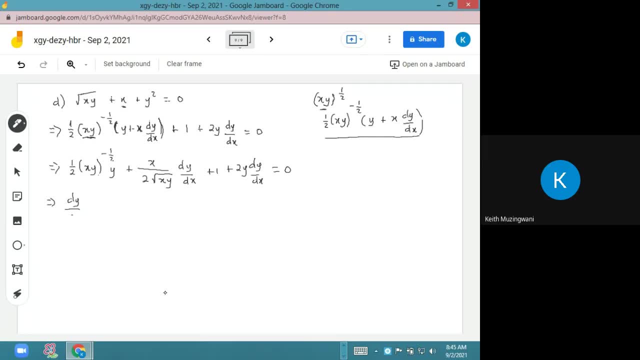 so we fact out dy dx, so we have x over 2. the root of x, y and plus 2y is equal to. we take one, the other side as a negative, also negative half, x, y to the negative half, multiplied by y, and then divide by everything. so dy dx is equal to negative 1 minus half. 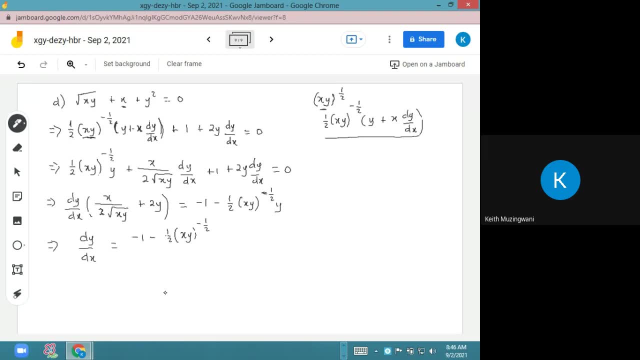 x, y to the power negative half y over 2 trava x over 2 root x, y plus two i. you can leave it in this form or you can decide to write a numerator as negative one minus y over 2 root xy. that's like we wrote the other one in the denominator. 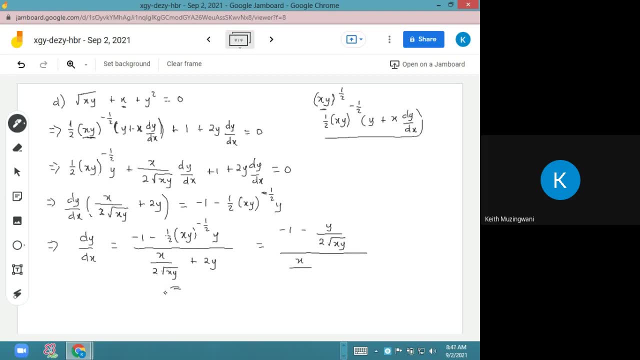 and then here I have x over 2, root xy plus 2y, like that. so, sir, there is no way they can give three functions multiplying. even if they give them as three functions multiplying, you take them in in two tools. okay, there's another example. okay, let me give one based on the functions multiplying. 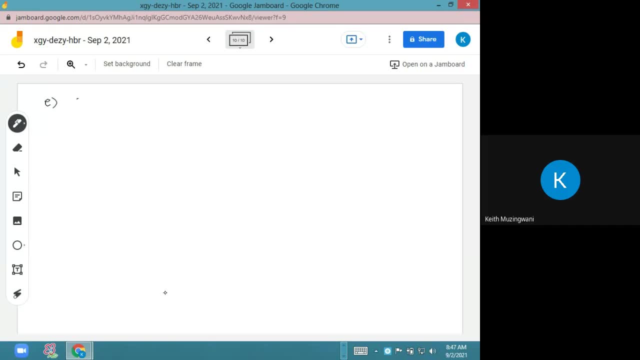 e. you can have x squared multiplied by x plus 3 to the power 4. multiplied by x minus 1 to the power 7, this is equal to y. x minus 1 to the power 7. x minus 1 to the power 7. 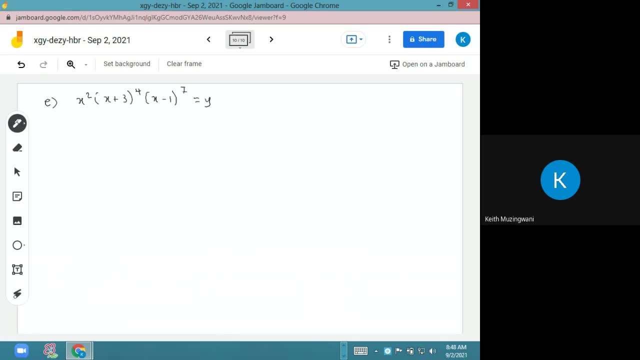 x minus 1 to the power 7 to differentiate. since there are three, you take them. you take u to be the first two and you take v to be the other one. you have issues differentiating u. you are going to have 2x and fix the other one because on differentiating you use product u. 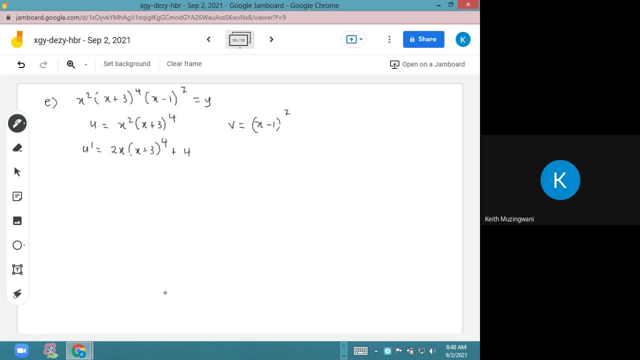 plus you draw. so we have f sub x, cub plus y. gave a approach we came up with means. you have to solve it this way: n to the power of 5, so v force to the power 3, that's x square. so now we draw x to the power 3. 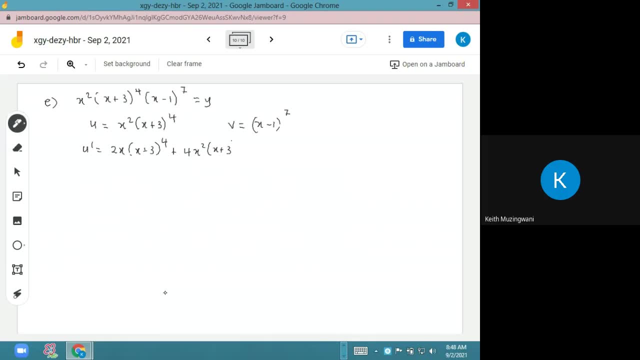 x to the power 5, then x squared, then x to the power 3 and 2 to the power 3, then x square. n to the power 3, n to the power 3, 1 to the power 3, x to the power 3. 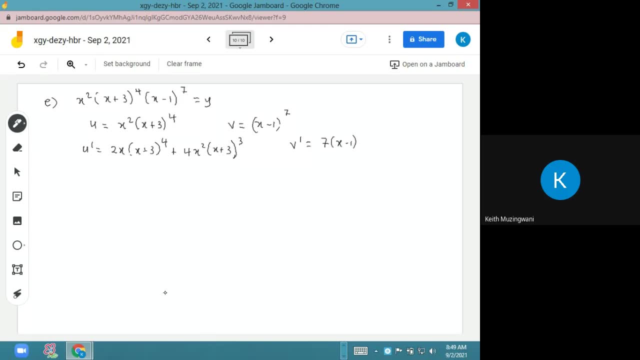 and we did this. so v to v prime will become the question one. is there anything else? we didn't answer, but we did next time the power six divided by one, and then gy, dx, as usual: y prime, v plus v prime, u, u prime is here, so you take it as it is. 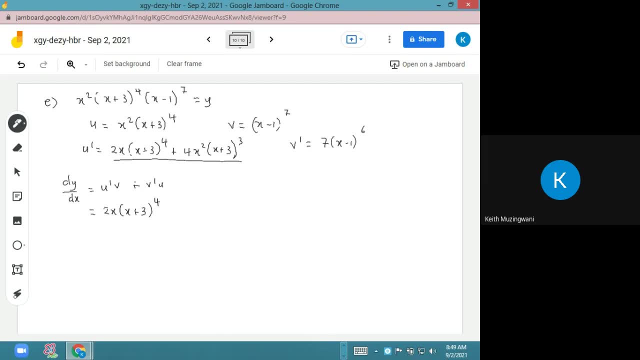 x plus three to the power four, uh plus plus four, x squared, x plus three to the power three. this whole guy multiplied by v, which is x minus one, to the power seven plus v, prime seven, x minus one, six, multiplied by x squared, which is u, x plus three to the power four. 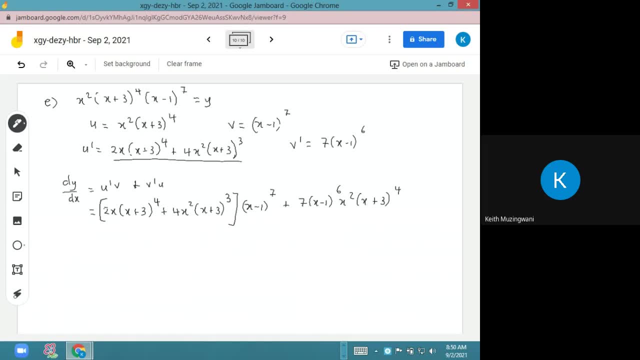 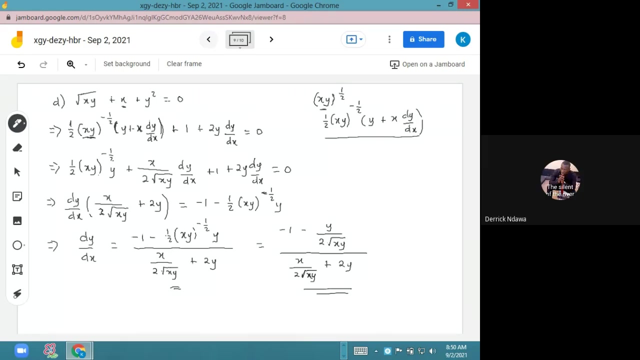 we are done, even if it was as a fraction. it's too separate in that manner. whether you are u or v and still carry on get to the solution. uh me have a question on part d. on part d, i don't know how you differentiated uh, x, y, which is in the bracket there you use. 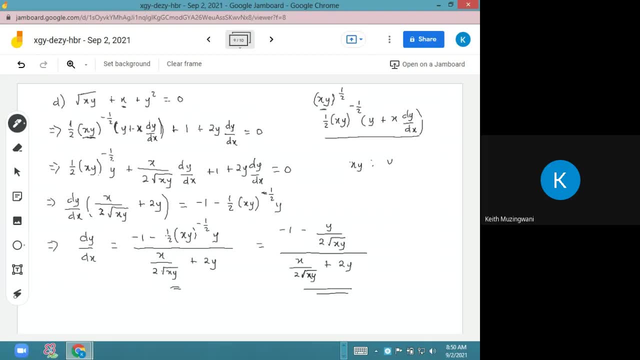 when you have x, y, you take it in the same way we take uv. so you let your u to be x and your v to be. when you differentiate u, you get one. when you differentiate v, you get 1 multiplied by dy, dx. but you know that 1 multiplied by anything is that thing, and then you write it as: 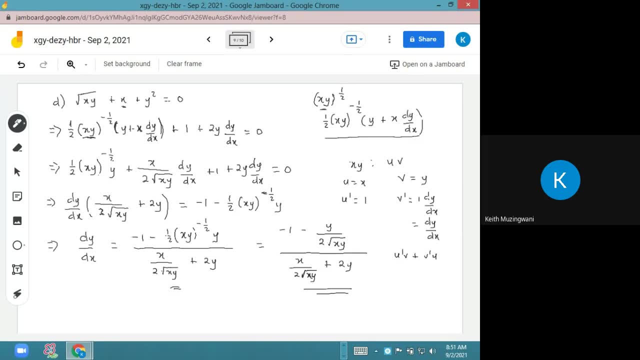 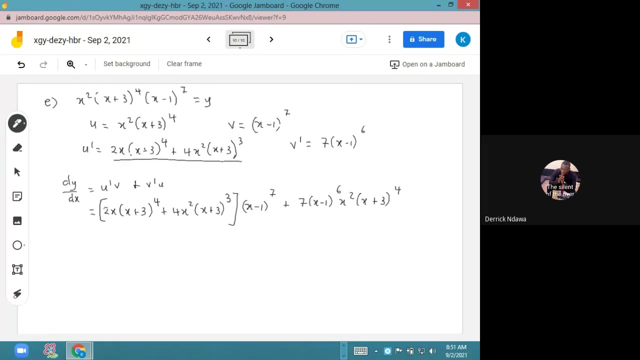 u prime v plus v prime u. so u prime is one, v is y plus v prime is dy, dx, u is x. so you have x dy the x. that's where we, that's where we have this inside. all right, thank you, sir. so um in the next session. 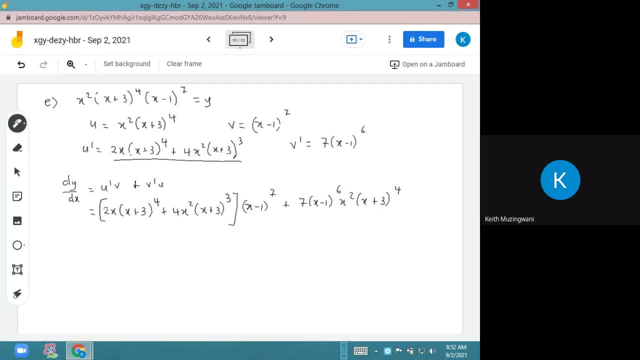 we'll be looking at that type. i gave you which you offered at the first question. second, functions of logarithmic functions. so how do you differentiate logs? how do you differentiate? so the next session will do the logs. that question i gave you and some trig derivatives. so if you miss, 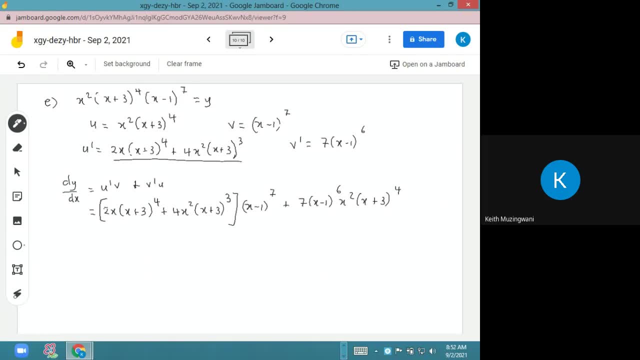 you'll miss a lot. i don't have to be missing, get a point. well, you make sure that if you miss, you watch the video, otherwise we have no time to test and i didn't give you the exam. i haven't forgotten. i want it now to include derivatives, so it will be given. so the agreement will be september. 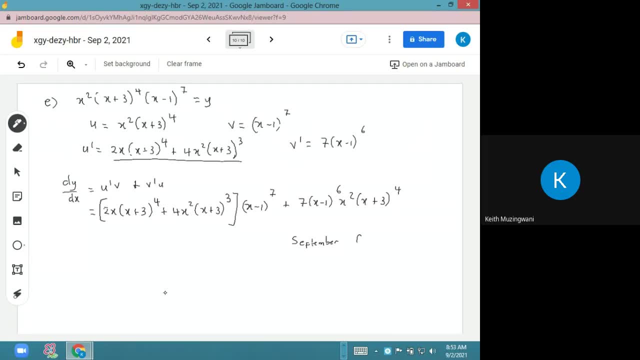 september, month end, exam one. here you can have difficulties. uh. october, month end, exam two. here. if your difficulties in one here need to improve, then the last exam will be november, which will be exam three. and november is our last month. december is for you to revise any days you'll be given. 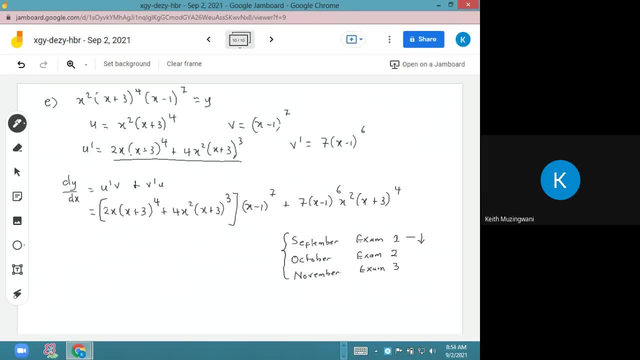 those are for you to revise, alone or with your friends, not to win, because i'm very sure that in these was, when you fail exam one, i'll burn you until you pass exam two, and i'll burn everyone until you charge the exam three. then i'll be at peace. 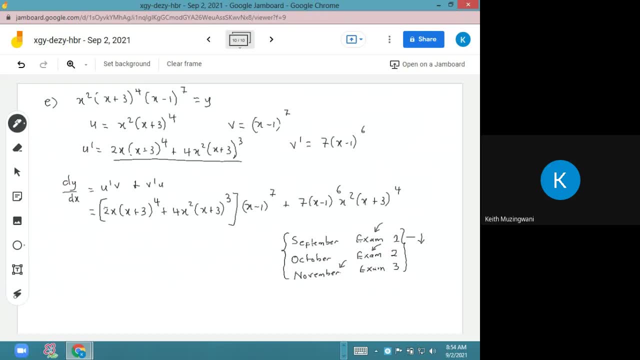 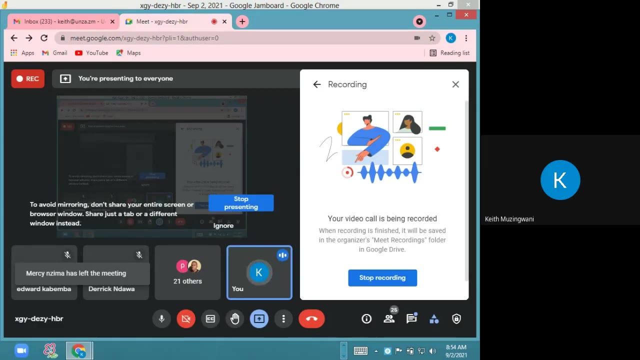 and i'll send you in the exam so that we end.